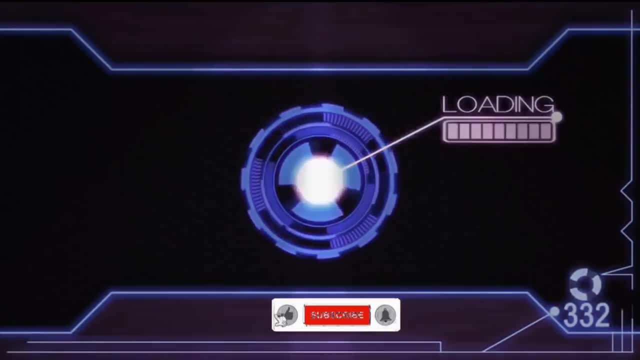 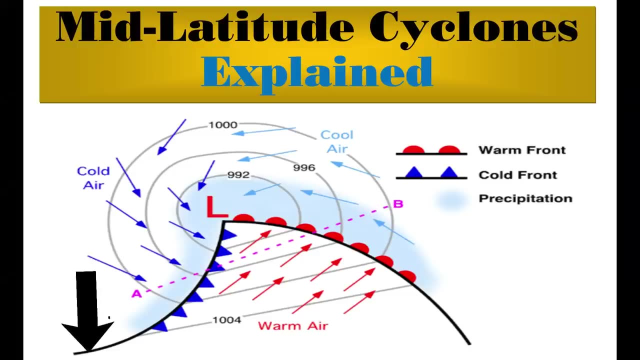 Please use the link below to get the notes, questions and other videos. Don't forget to subscribe, like and share to others for our daily new videos. Mr Godfrey, explain to us how do mid-latitude cyclones form And what are their impacts. 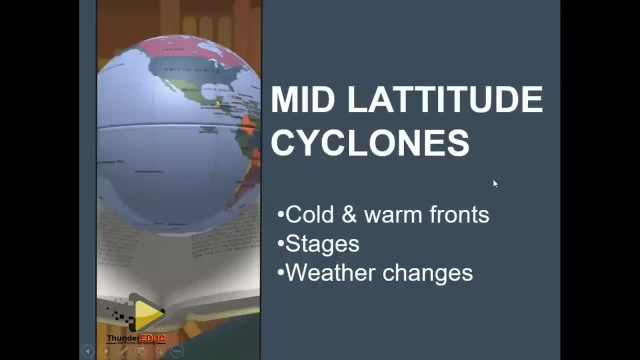 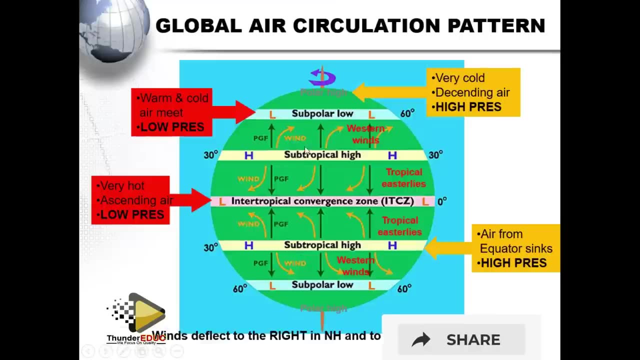 The mid-latitude cyclones, like the way the name is mid-latitude cyclones. We quickly go back and look at this. okay, It's called mid-latitude. These are latitudes, These are latitudes. These are latitudes. What are latitudes? Those are magic lines that are drawn from west to east. 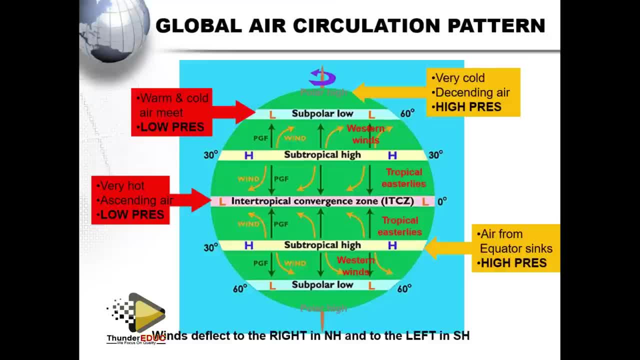 increasing. In the northern hemisphere it increases to the north. In the southern hemisphere it increases to the south. When you look at these lines, you draw this, you draw this, you draw this one. So when you look at it, we have this segment here and we have this segment. Where is the mid? 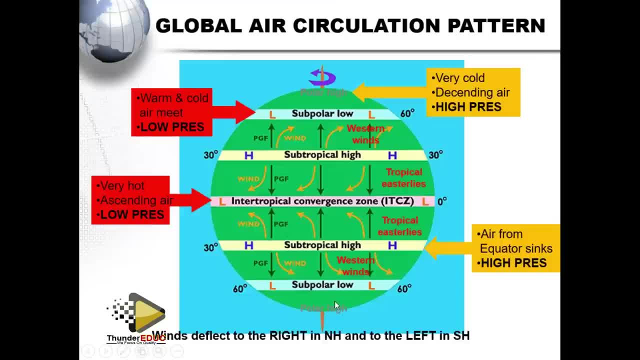 The mid is here, So this one is the mid area of the southern hemisphere. The same way, in the northern hemisphere we have this segment. here We also have this segment. This is the mid. So that's why they call it mid-latitude cyclone, meaning that it is basically occurring between 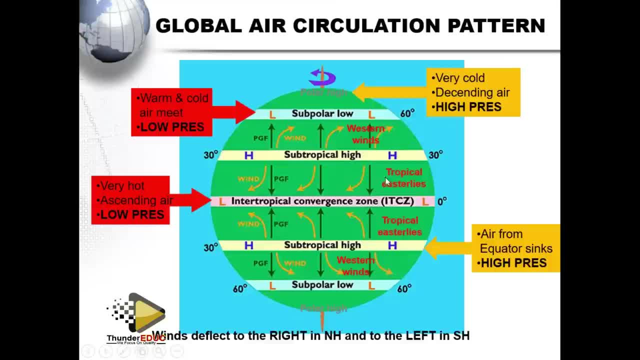 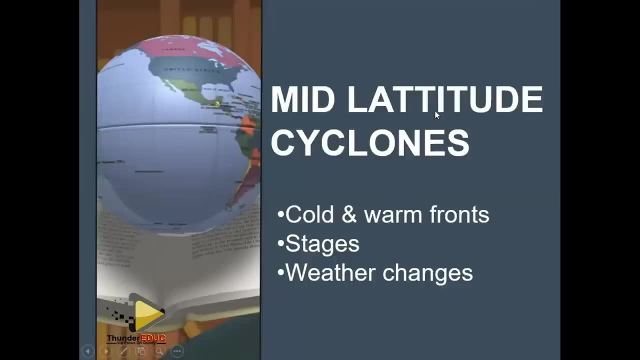 the mids of the latitudes. So it is occurring between 30 and 60 north and south of the equator, the same way north of the equator, the same way 30 and 60 south of the equator. okay, So it's called mid-latitude cyclone. But you must not forget learners. 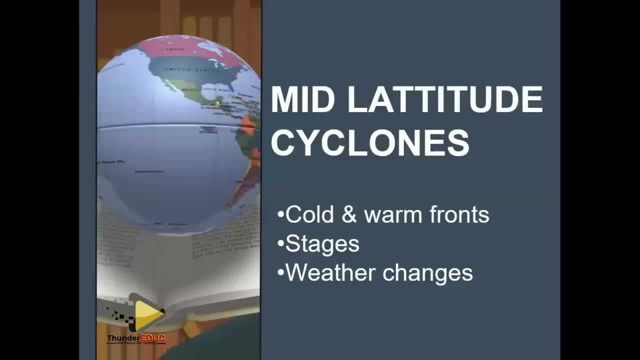 that mid-latitude cyclones are also known by different names. For example, it is known as a temperate cyclone- okay. It is known as frontal depression- okay. Extratropical cyclone. Sometimes we miss that one mark in the exams because you're forgetting the name of the cyclone, So you're. 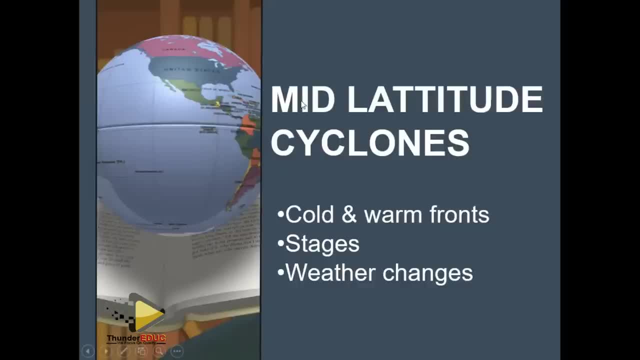 forgetting the name of the cyclone. So you're forgetting the name of the cyclone, So you're forgetting those simple names. But let us look here. It's called mid-latitude cyclone as it is found within the mid of the latitudes And the cyclone is basically low pressure When you go. 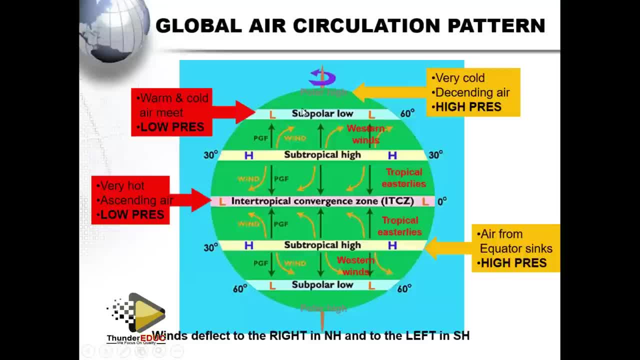 back to this diagram. you are going to find out that we said the mid is here And this is where you have a low pressure, So it forms here at the subpolar, basically at 60.. The same way here it is here at the subpolar, at 60,. okay, That is where it is found. 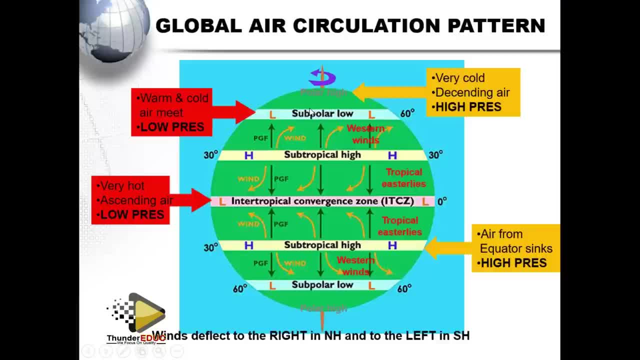 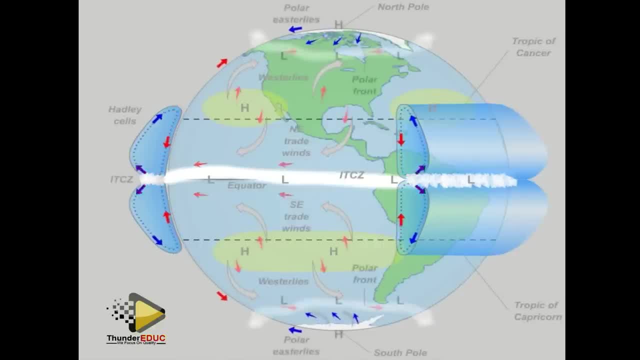 But what is going to happen? That it forms because we have got the westerlies and we've got what The easterlies from the other side Remember. this one is called the polar easterlies and this one is called the westerlies. These ones are warm as it is coming from the subtropical. These ones are: 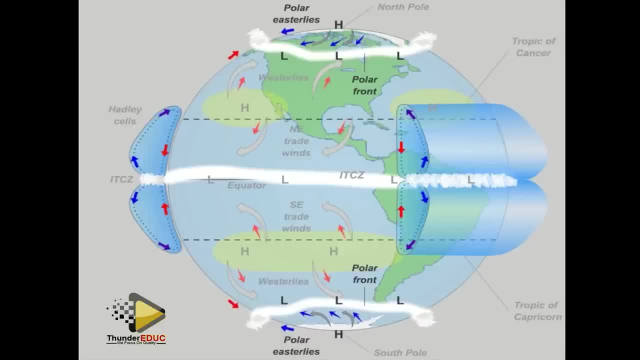 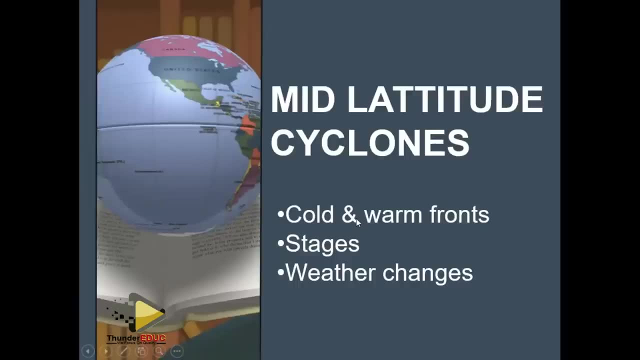 cold as it's coming from the poles, okay. So we must note that cold and warm fronts here exist at the mid-latitude cyclone. What you must note is that when we talk about mid-latitude cyclone, the first thing that should come into your mind or in your head is that cold front and the warm 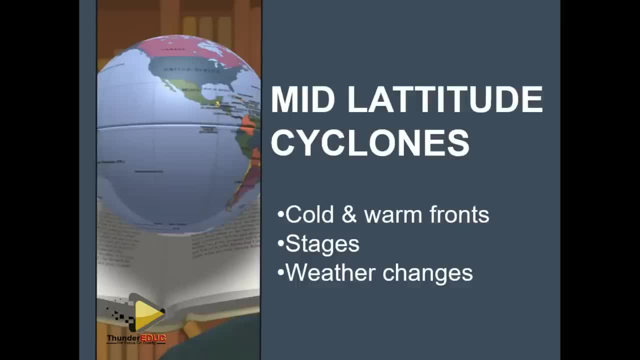 front. how do they exist? That would be the next thing you are going to look at. So we are going to look at the cold and warm front. We are going to look at the stages and the weather changes that come in or that exist because of the cold front. So here we go. What? we must note that? what is a 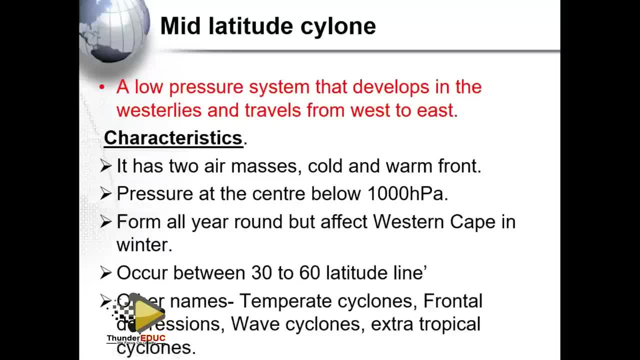 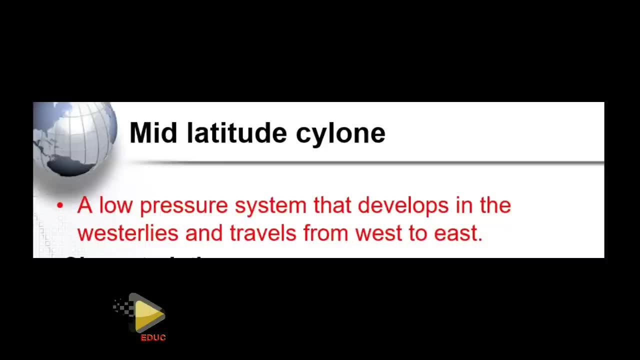 mid-latitude cyclone. What does it mean? You must understand. We say that if you see a typhoon, you forms 30 to 60.. you must understand that the mid-latitude cyclones are low pressure systems. it is a low pressure system, if you must note that it is a low pressure system that develops in the 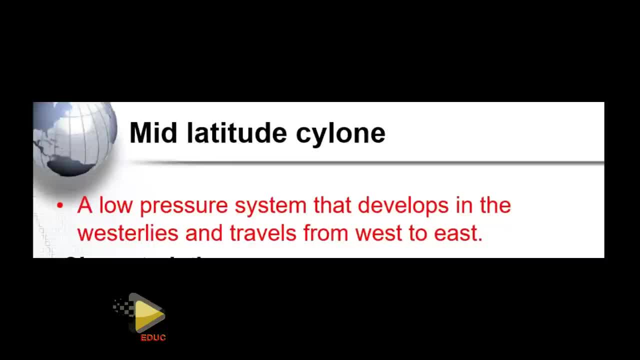 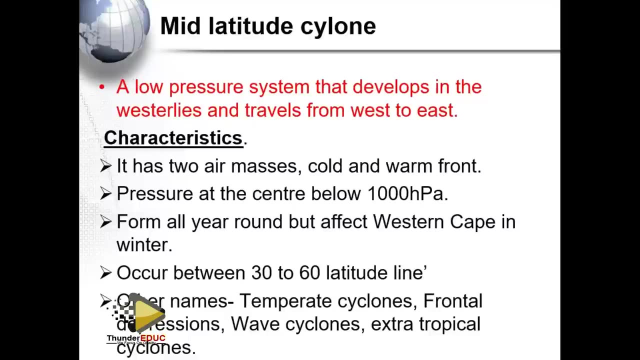 westernies, traveling from west to east. sometimes. i always want to add on that it is. it develops because of, um, the polar easterlies and the westerly winds, okay, so you must know that it's a low pressure system that develops in the westernies, okay, and it travels from east to west. 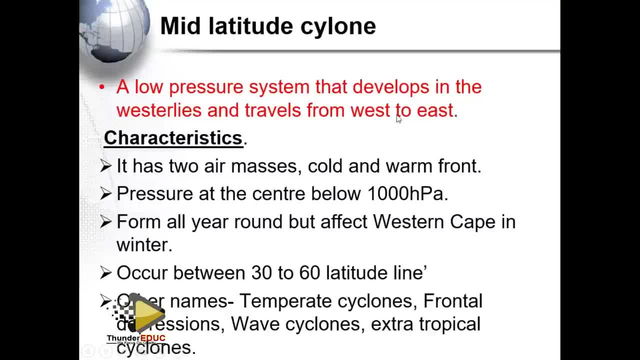 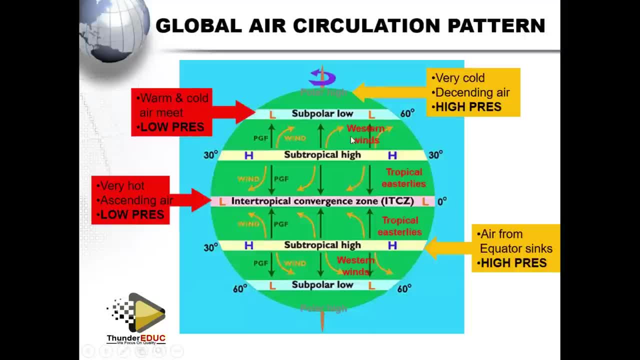 you must understand why is it traveling from east to west? it is traveling from east to west because it is part of the westernies. remember we said that western winds. what happens to the western wind? they travel from west to east, since it develops here between 30 and 60 and these winds are moving. 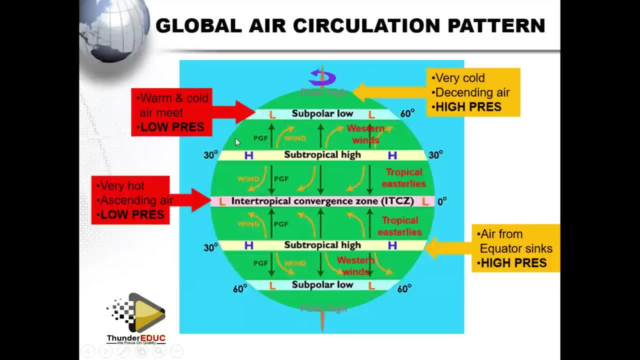 from west to east. so the cyclone itself is also going to travel from west to to east. that's why we say it develops within the westernies traveling from east or providing from west, sorry, to east. you understand the same way. here it is between 30 and 60 traveling from west to east, as it is part of. 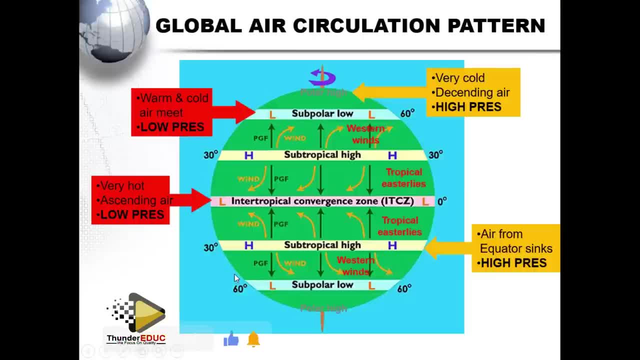 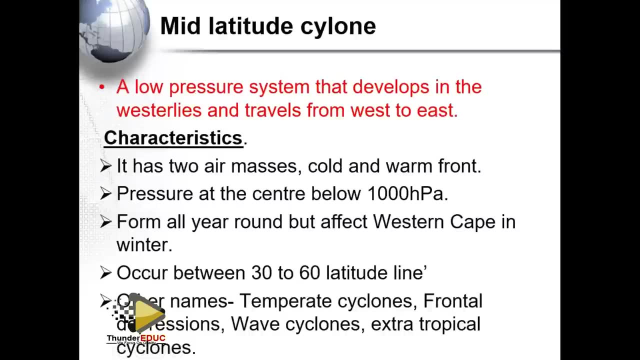 the westerly belt, which is moving from um west to east. okay, what are the characteristics? what can you look at? what features can you tell? what can you look at to say this is exactly immediately cycle. please learn us understand that. the characteristics clearly tells us that this. 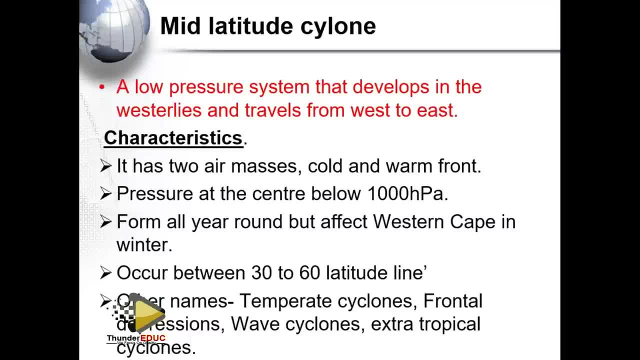 is a tropical cyclone, this is a middle-aged cyclone, and so on and so forth. therefore, since you are looking at the media, recycling what happens here, it has got two air masses. that is, cold and warm front. it has got two air masses. these air masses results into the development of 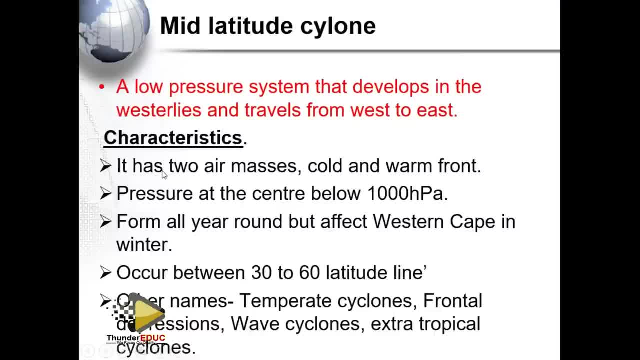 different fronts. remember we said that one air mass is coming from the polar regions, which is cold, and there's another air mass that is coming from um, the, the, the subpolar region, which is the westernies, and it is warm. this results in the development of of us having warm front and 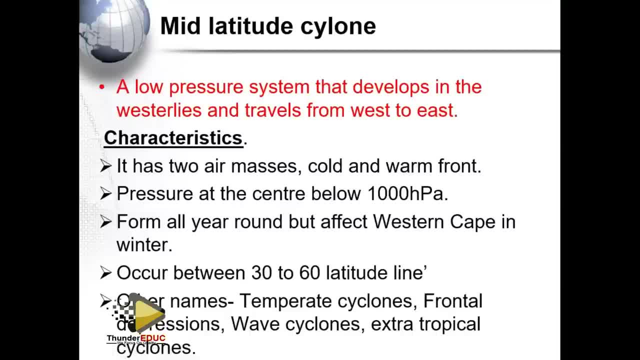 the cold front. in other words, when you look at immediately cycle, you know that we shall have um, we shall have the cold front and the warm front developing. therefore, we also note that, since it is known as a low pressure, remember when we are looking at, the first thing that we looked at at. 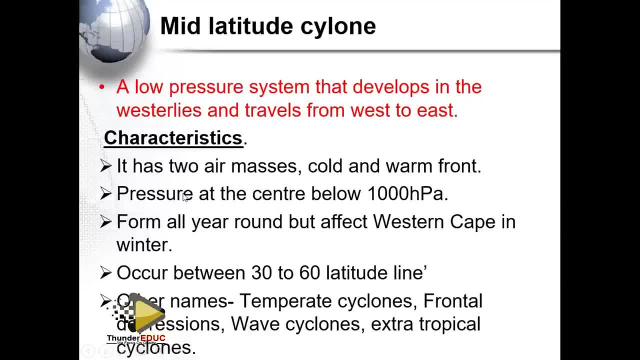 the beginning we said low pressure. pressure decreases towards the center and therefore pressure must drop below a thousand hectopascal. we said hectopascal are the si units of pressure which is measured on a. so pressure at the center is always below a thousand hectopascal, decreasing towards the 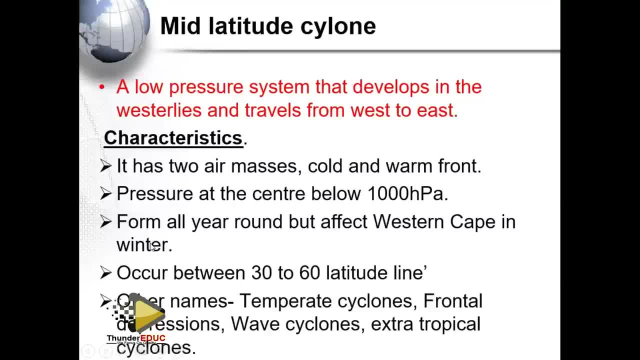 center. that's why it's called a low pressure, and it also says it forms all round, all year round. but it affects western cape in winter. we know why do we say it more. it it forms all year round. remember this system. it moves um with the apparent movement of the sun or the itcz. what happens is: 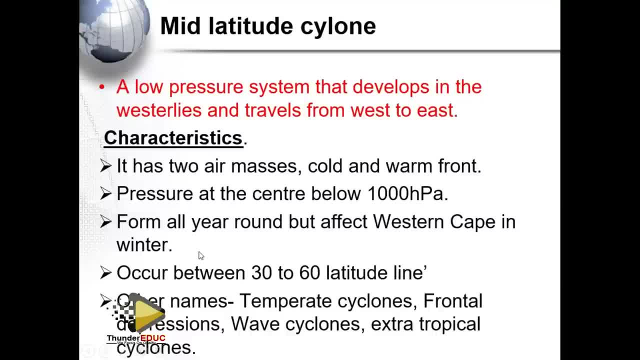 that if it is winter in the southern hemisphere, the system moves close to south africa, but if it is summer in the southern hemisphere, the system is forced to move further away from south africa. that's why we say it formed throughout the year. the only fact that it only affects south africa. 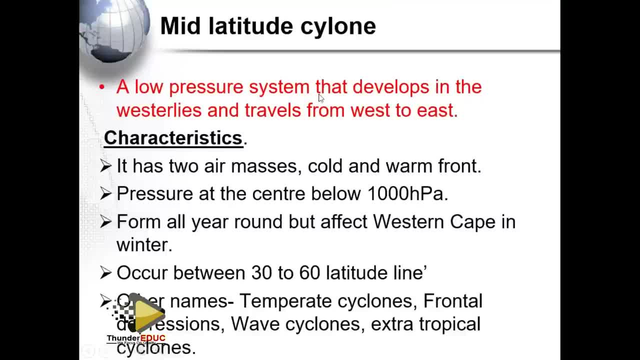 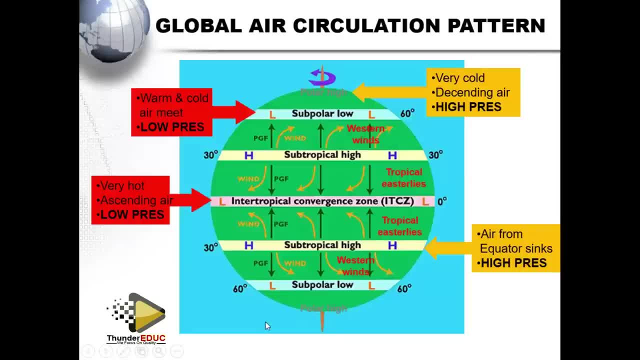 only during winter, but it is occurring throughout the year. all right, then We also say that it occurs between 30 and 60.. We have noted it. It's a mid-latitude cyclone midway. The mid is here and the degrees are here. 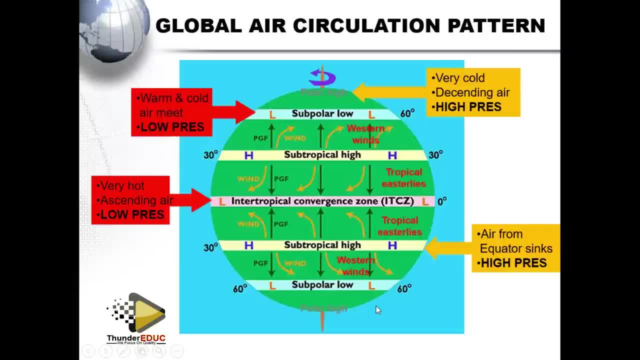 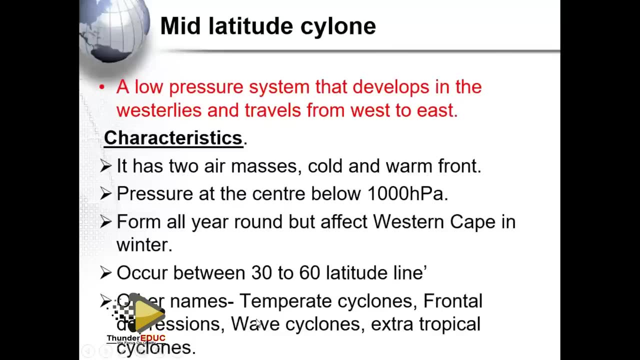 Latitudinally it is located between 30 and 60 north and south of the equator. We go ahead and say the other names. Like I said, it's known as a temperate cyclone, frontal depression, a wave cyclone. 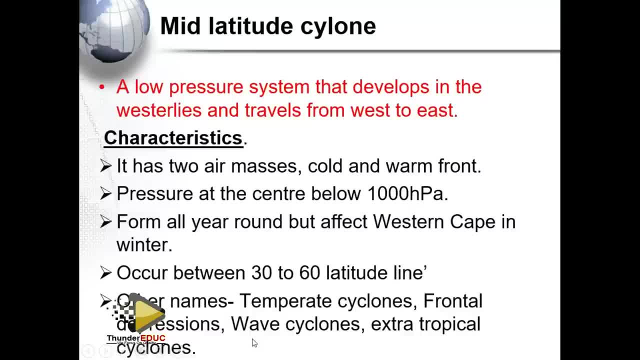 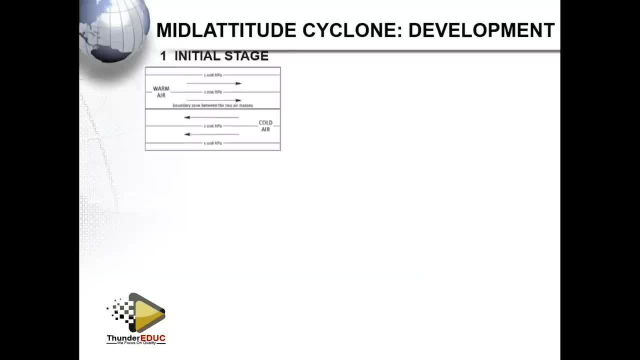 extra-tropical cyclone, and so on and so forth. So those are the names that can be used to refer to a mid-latitude cyclone. okay, Now we must know that it does not occur once A mid-latitude cyclone takes stages. 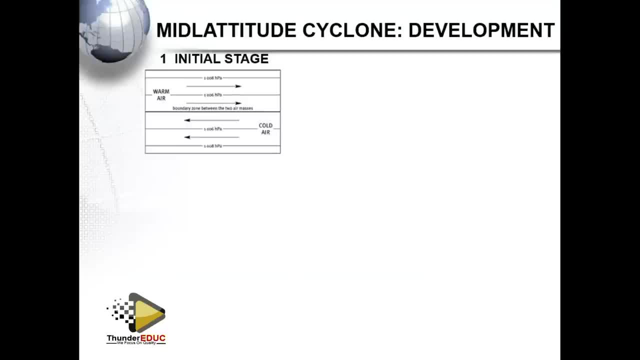 It occurs in different stages. The stage is the first one, that's as the first stage is what you call the initial stage. Remember, on our diagram, This way we are going to focus specifically Or mainly on South Africa, And in South Africa we know that the cold air or in the southern hemisphere, 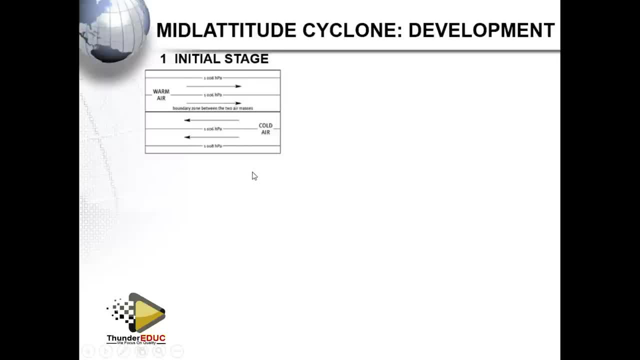 the cold air is in the south, The warm air is in the north, And these two air masses are coming from different directions. okay, So the point here where the air masses are going to meet, or they are going to converge, is what you call a polar front. 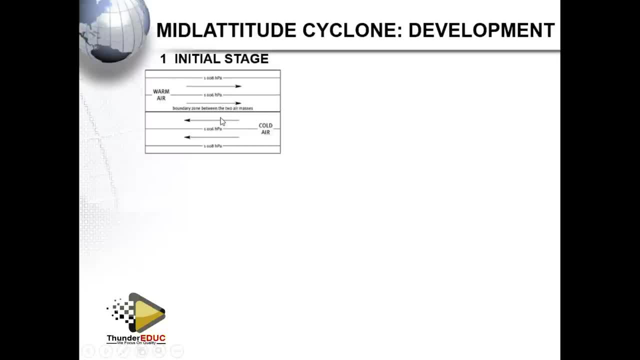 But what you must note, that the pressure in the initial stage is still high Because the cyclone is just starting to develop. The pressure is still high. The pressure is still high. The pressure is still above 1,000 hectopascals. 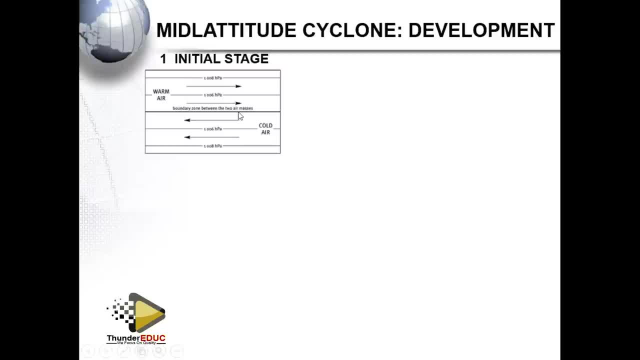 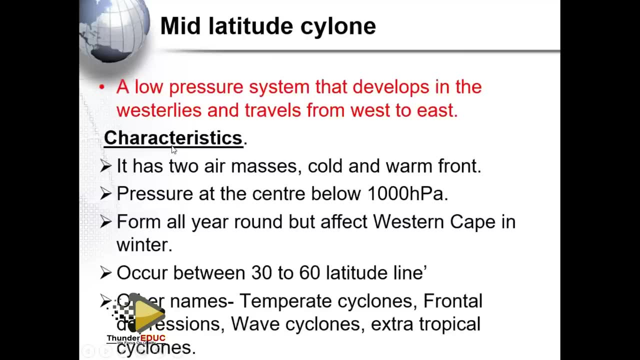 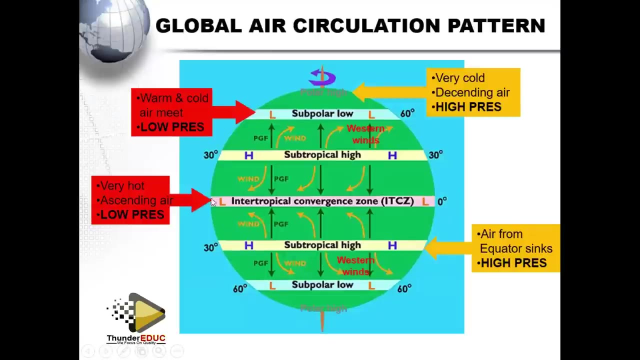 That's why you see, close to the boundary zone that is separating the two air masses, Pressure is still above 1,006 hectopascals. We quickly go back to the diagram. I will basically use this diagram so much When you look at this. let us first of all ignore this northern part. 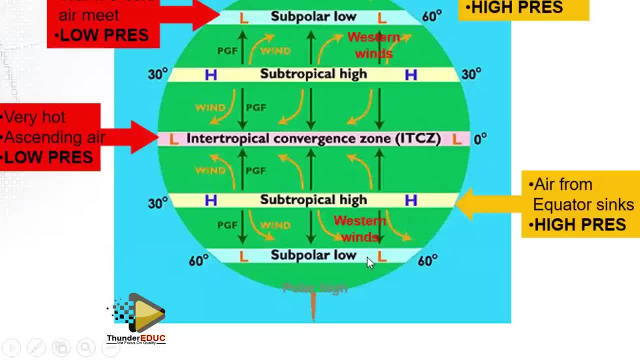 Let us look at the southern part. When you look at the southern part, this is the southern hemisphere. We know that there is air that is coming from this other region, which is the polar eastern, And its meeting point is here. So, as it is coming from the poles, this one at the bottom is going to be cold. 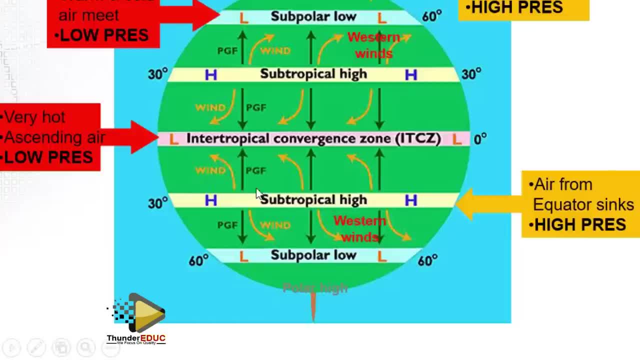 We have this one that is coming from the subtropical. So, since it is this subtropical, it's close to the equator. it's a bit warmer compared to the poles. Therefore, we have the northern part, which has got warm air. 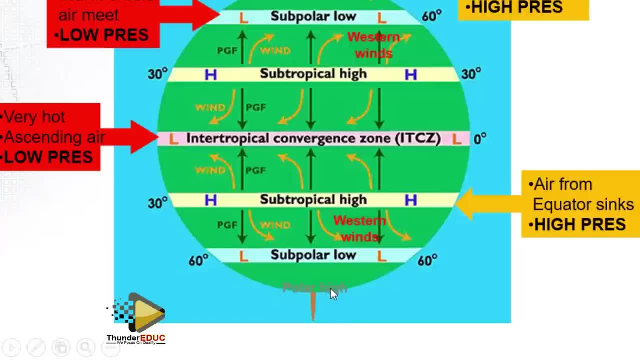 So we have the warm air and we have the cold air. Remember this one. It's coming from this way, It's meant to go the opposite direction, and this one is meant to go the other direction. So the reason this one is called Easter is so because it's called Easter is it moves from east to west. 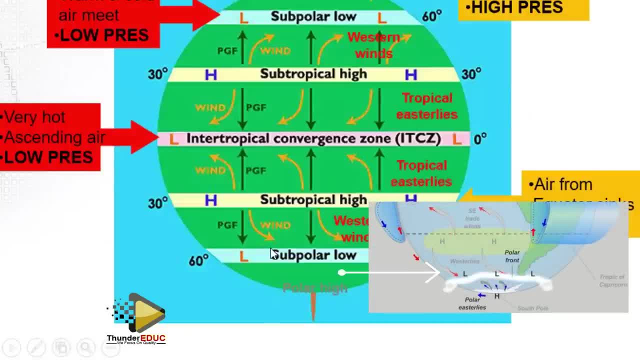 Therefore it is meant to be moving like this to the other side, And this one is meant to be moving from the west to east. Therefore it is moving like this, So it's just bypassing each other at the sub polar low pressure here. 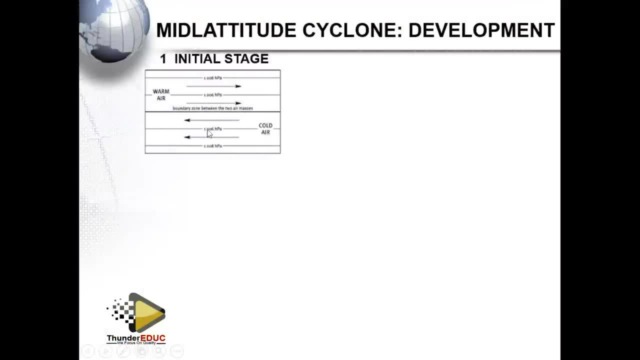 So, in that case, the way it is here is the way it is reflected There, The other side, warm air above, passing from. remember it is westeries from the west going this other side. These are the Easter is from the east, going this other side. 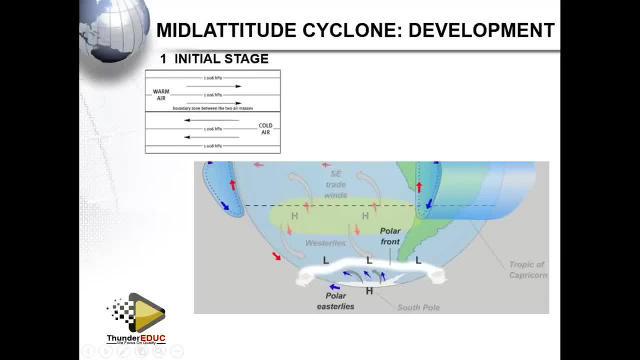 That is the initial state. What you must not do The initial stage is that it is sometimes referred to as a stationary stage because boundary is not moved at all. Okay, That's why we call it the stationary stage. We've got the second stage. 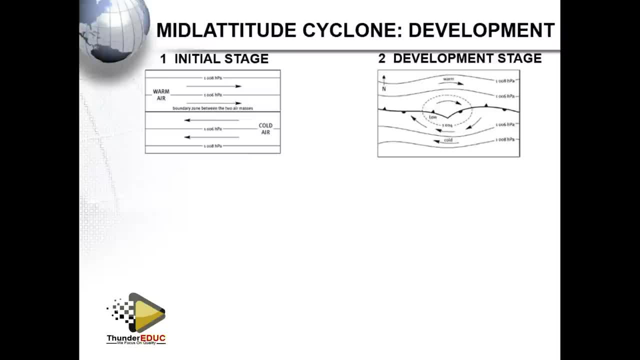 The second stage is also known as the developing stage or the development stage. In other words, Some other books will call it a wave stage. In this case, pressure starts to drop and a wave develops and therefore the rotation of the wind. at a low pressure it starts and therefore it rotates in that clockwise direction. 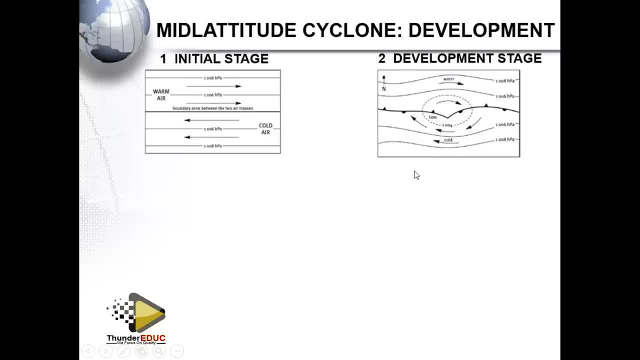 Remember, we are looking at the southern hemisphere. We said: in the southern hemisphere air circulates in that clockwise direction. That's what. that's why the arrows are pointing in this direction, southwards. Therefore, this is the northern part, This one. 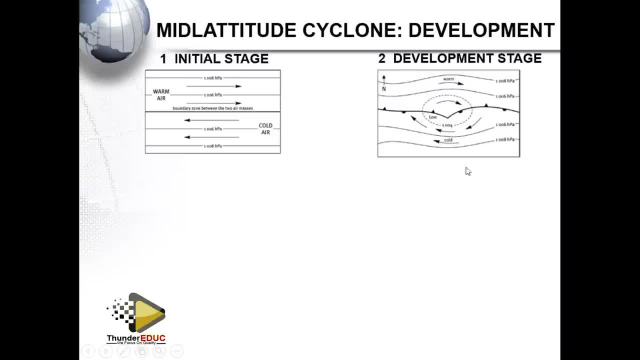 This one is coming from this way. This one is coming from the east and therefore it is rotating at a low pressure that is starting to develop in that clockwise direction And in this case, a wave develops and you will see that the fronts are also starting to develop. 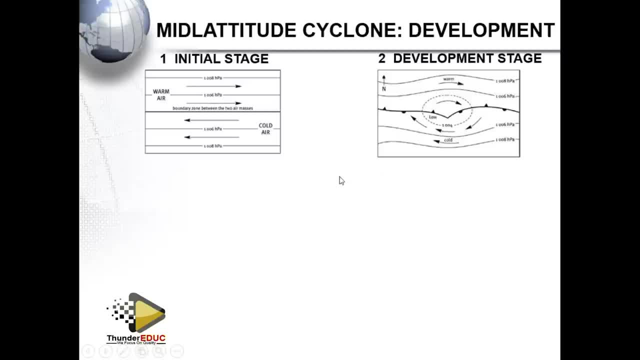 Okay, And that is the apex. The pressure is dropping to below a thousand hectares per square, But it is still high. So we got the second, another stage, which you call the mature stage. In the mature stage, pressure drops further, below a thousand hectares per square. 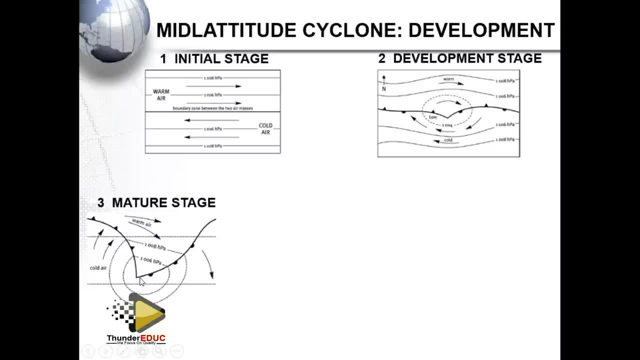 So therefore, here it's going to be below nine, maybe 984 hectares per square, A cold front and a warm front is visible at this stage. So what happens here? How do you notice that this is a cold front and this is a warm front? 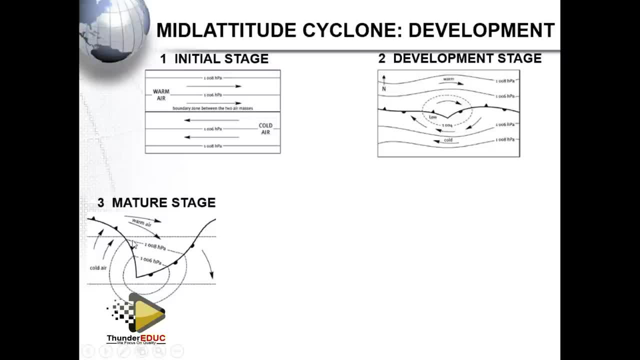 A cold front is represented with a triangle. Okay, A warm front is represented by a semi-circle. So what happens is that behind a cold front is a cold sector and behind the warm front is a warm sector. What you must note that this cyclone is moving from west to east. 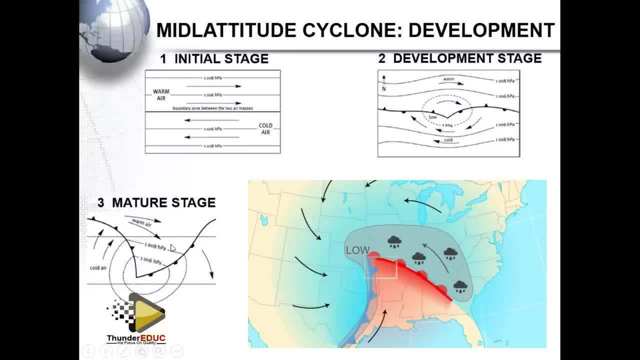 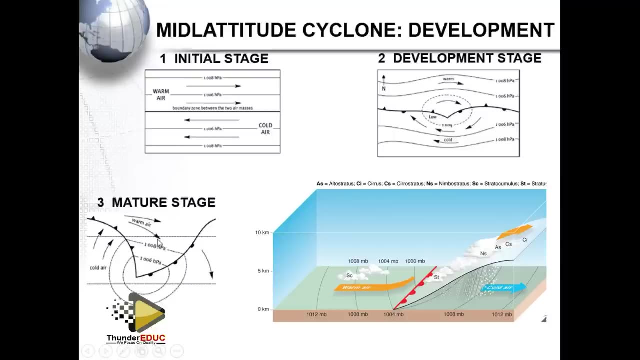 So it's going in this direction. while the air is circulating in that clockwise direction, as it is rotating, the sectors of warm sector and the cold sector- Okay Okay- becomes clearly visible And therefore, because it is visible, the warm sector is developed here. 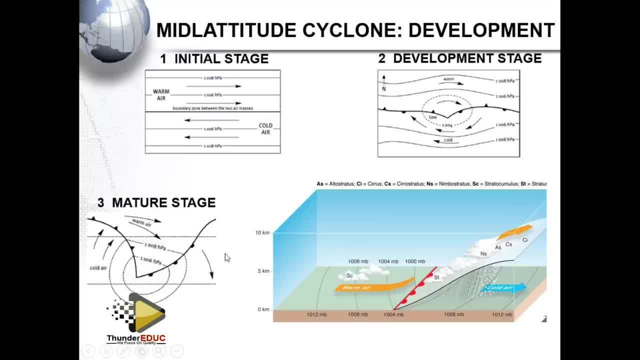 It is behind the warm front. So this is the warm front here And here is the cold front. Therefore, behind it is the cold front, The whole of this sector here is the cold sector. Okay, So the air behind the cold sector is cold And the air behind the warm sector is warm. What we must note that 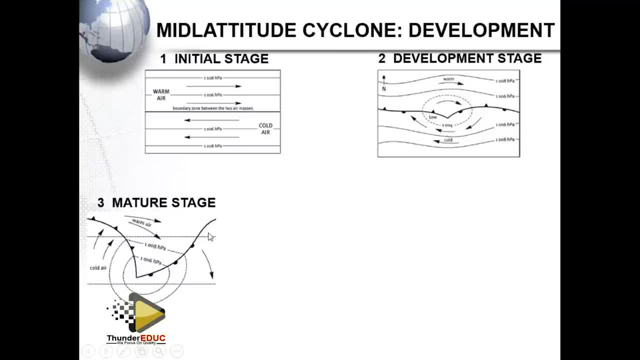 this is a mature stage. And the mature stage, cold front and warm front- are visible. They are easily identified. Okay, We go to the next stage, which we call the occlusion stage. So in this occlusion stage, we must understand that cold air is heavy and denser, Therefore it moves faster. 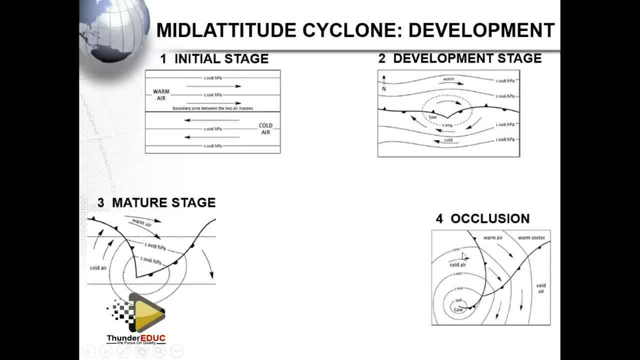 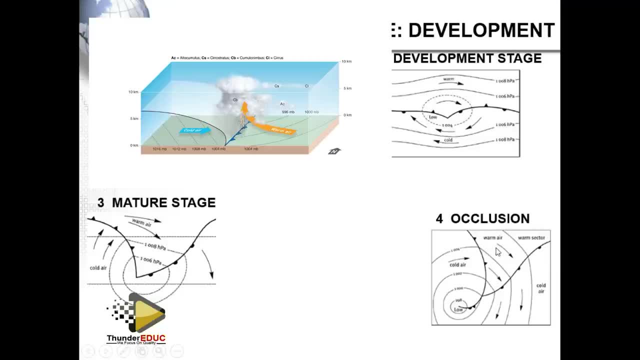 than the warm air. This is going to force the cold front to catch up with it, to catch up up with the warm sector, narrowing the space that was occupied by the warm sector, as it is pushing the air, the warm air, outside the cyclone. so meaning that, as this one catches up with the 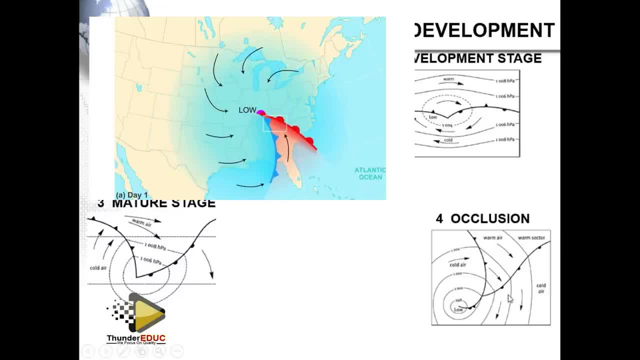 warm sector. we are going to see that at the apex the two symbols are going to be um represented. so these two symbols that are represented, it is a symbol for the warm front and the symbol for the cold front. the triangle is the cold front. the semicircle is um. the triangle is the cold. 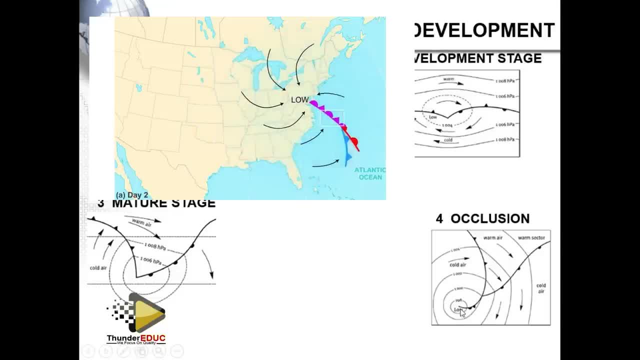 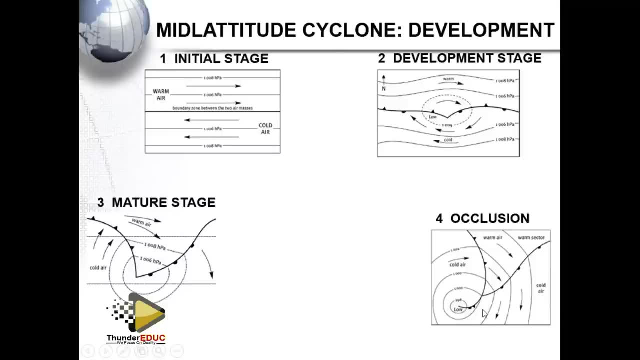 front, the semicircle is the one front. therefore, this is what you call the occlusion front. so in this occlusion front, um, in this stage, the occlusion, it results into the development of the occlusion front. so we have the cold air behind the cold front, in the cold sector. 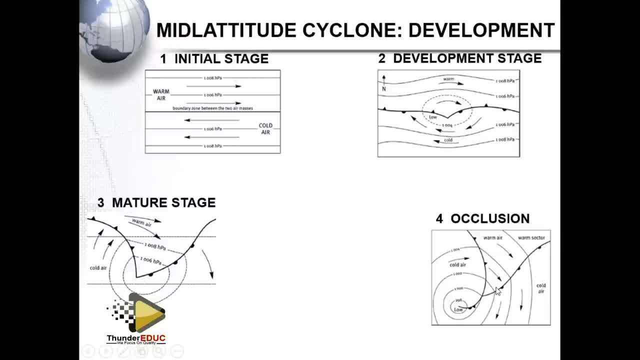 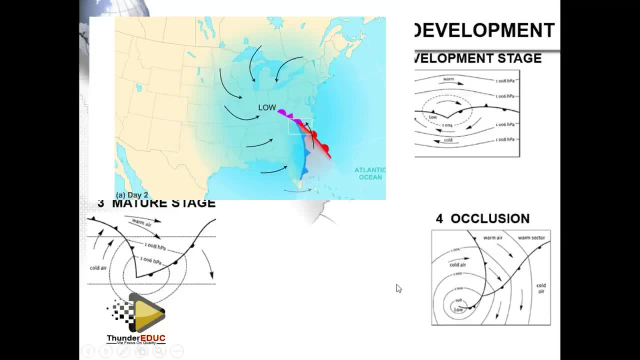 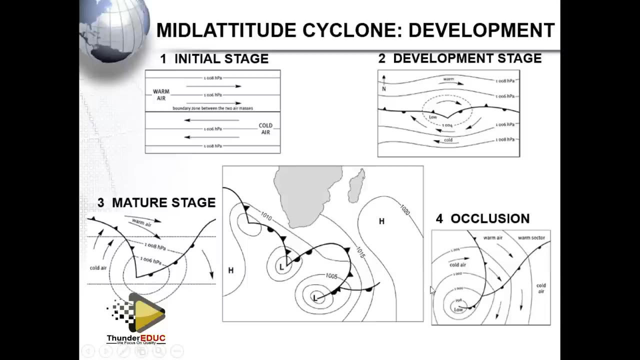 we have the warm air in the warm sector that is behind the warm front, and this is what you call the occlusion stage. Then, in this case, when you look at these two stages, there is a characteristic that we did not mention, That characteristic that 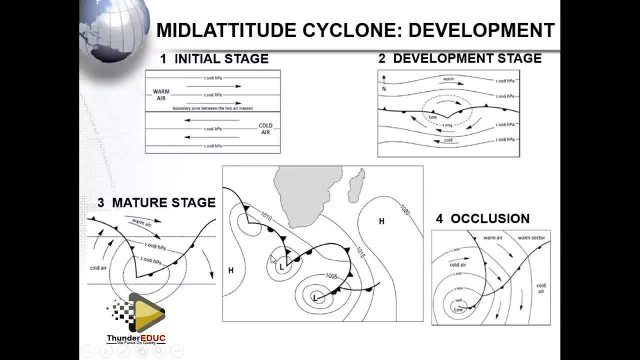 we didn't mention is that mediatory cyclones occur in families. We have them occurring in families, That is. there is one here, there is this one here, there is this one here. What is a family of a mediatory cyclone? These are series of mid-latitude cyclones and when you look at it, 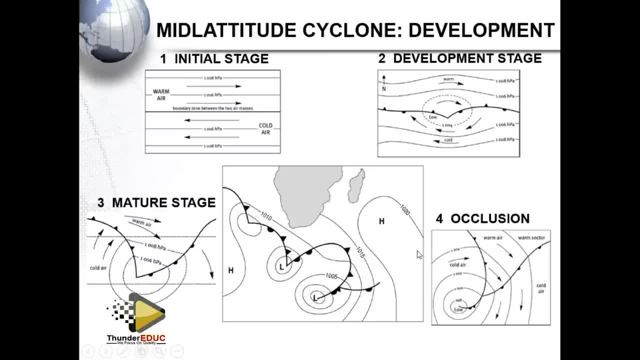 it is moving from this other side of the west to the side of the east. Remember we have a high pressure here and we have a high pressure here. Sometimes this high pressure is also known as a blocking high. It is blocking this cyclone from going into the other side, so that will force it. 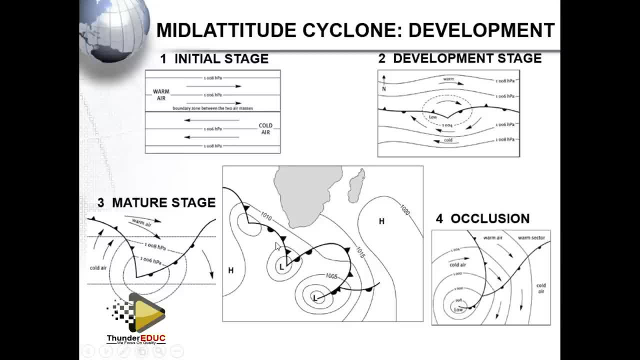 to move, so that it can move this other side, but still in the western direction. So what we must understand is that the cold front on this other side there is also a cold front here. there is a cold front here, there is a warm front here. It is moving from this other side to this other side, If you notice. 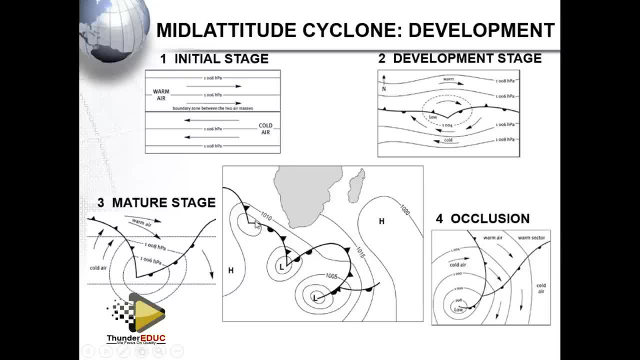 let me say: this one is A, this one is B, this one is C. Of the three, which one is mature? It's going to be that this one, A, is going to be mature. Why is it mature? Because this system is. 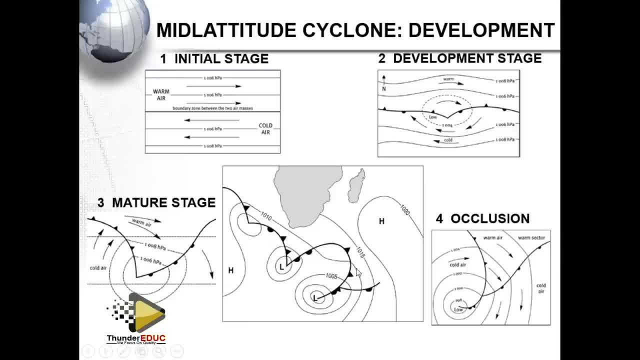 moving from west to east. There are four. It simply means that even this one was once in the west, but because it is moving the other side, it is moving in that direction. Actually I can. this one is depicting almost the stages Here. it 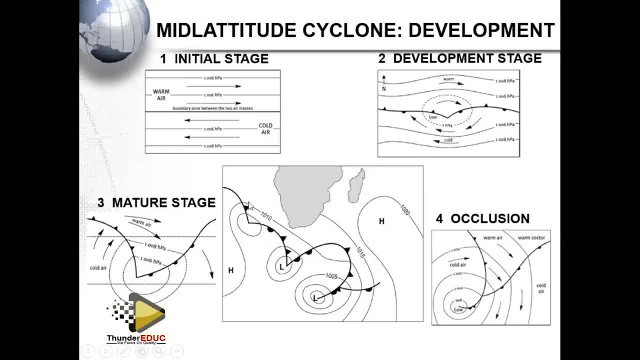 is the initial stage, okay, when it is just starting to develop. Actually, this one could be the developing stage when it is just starting to, a wave is just starting to develop. Then this one is the mature stage. You can see that the cold front and the warm front is visible, and here you. 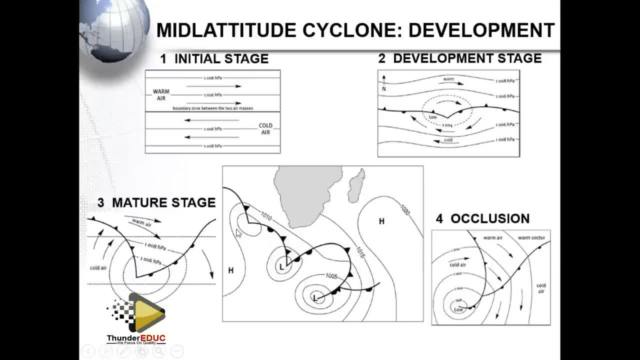 have the occlusion stage, Meaning that as you move away from the west to the east, the cyclone, the stages are starting to develop And therefore there is a nasty stage which you call the dispatch stage. Okay, the last stage will. 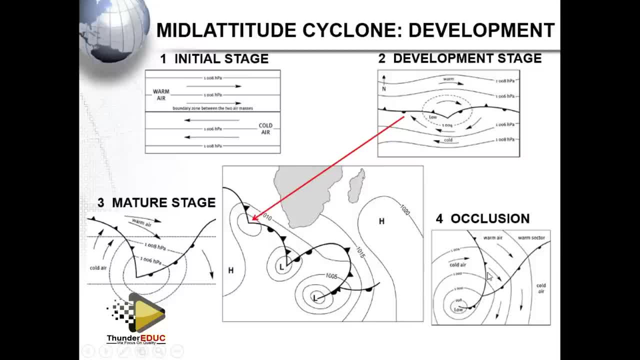 be called the dispatch. what The dispatch stage? What happens? that, as warm air is pushed away from the ground, the ground is going to be only occupied by the cold air. So that means the cyclone starts to die. So this one is what we say the developing stage. 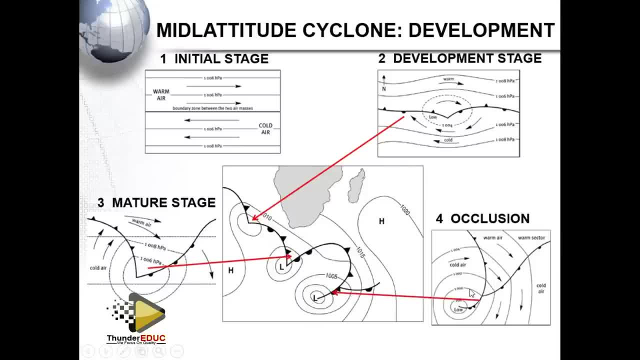 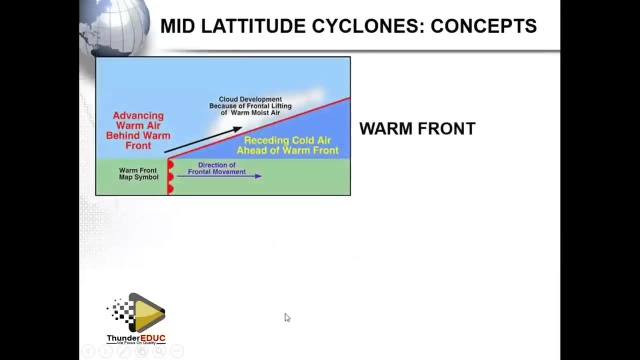 This one is the mature stage. This one is the occlusion stage, as it is indicated by the symbols on a diagram. Okay, So the whole of this is called a family of mid-latitude cyclone. Alright, now we must note that the occlusion stage has got two fronts. 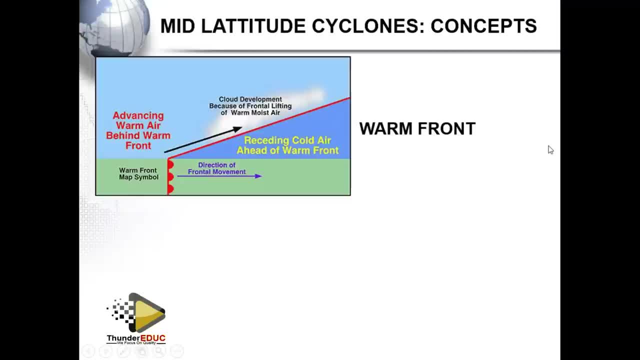 Okay, we have the warm occlusion front and the cold occlusion front, but the warm occlusion occlusion front is has got the characteristics of the warm front and the same way, the cold front, the cold occlusion, has got the characteristics of the cold front. this is how the cold, the warm, 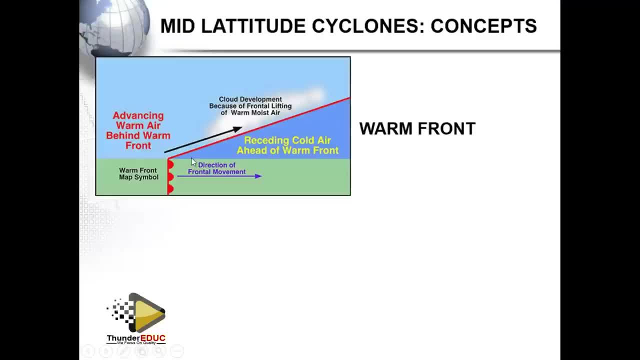 front is going to look like. what will happen? that when you look at this line, this line is gentle, okay, which is a bit different from this one. when you look at this one, this one is, uh, stiff, this one is gentle. what happens is that as warm air, as warm air reaches this point, it is forced. 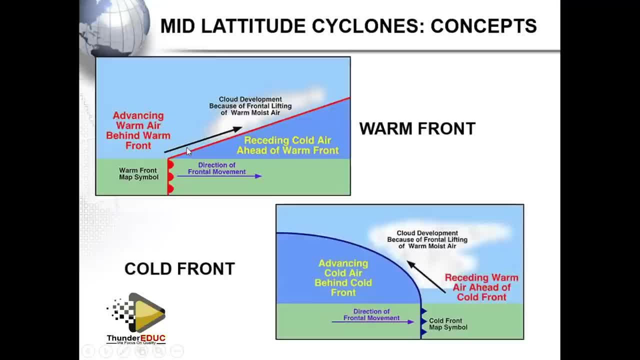 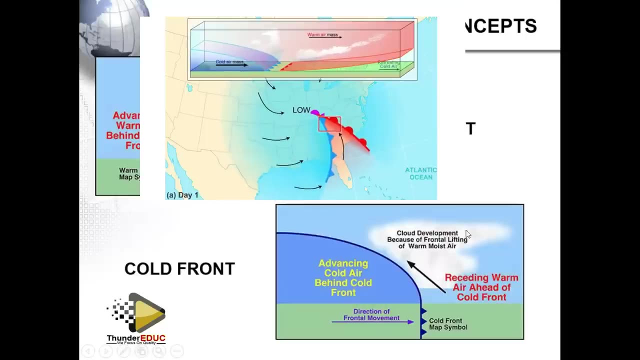 to rise, and it is rising at this point, meaning that if these two are put together- one is here, another one here- the warm air is going to rise and then, as it rises, it is going to result into the formation of clouds here, just on the cold front. so these clouds would 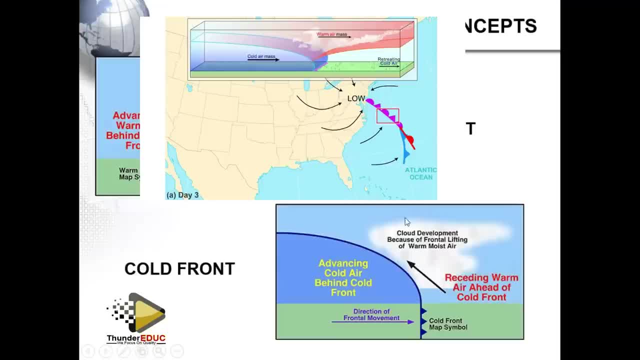 result in this kind of temperature and this is called the rice, because the rice doesn't move. this is called the rice doesn't move because the rice doesn't move, because the rice doesn't move out into the formation of heavy rainfall and therefore heavy rainfall will be experienced on the cold front. 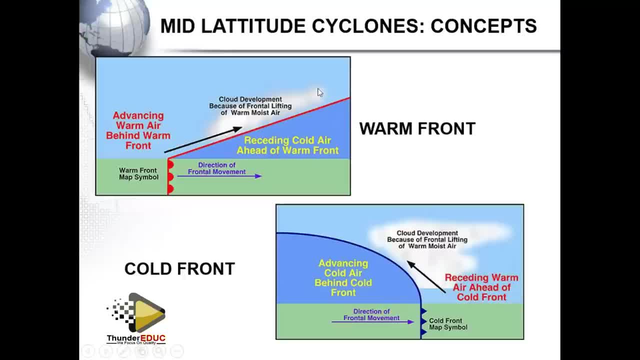 But here we have got some kind of clouds that are going to develop. Actually, I normally use the word cairn, which is karas clouds, ultrastratus clouds and nimbostratus clouds. These are the clouds that develop here. 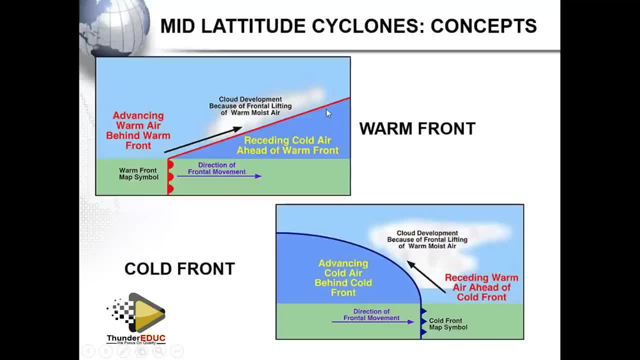 When you look at the shape of the clouds here they are light and a little bit growing longer. Why are they growing longer here along the warm front is because of the fact that this wind- there is also some air that is moving along this, which results into it. 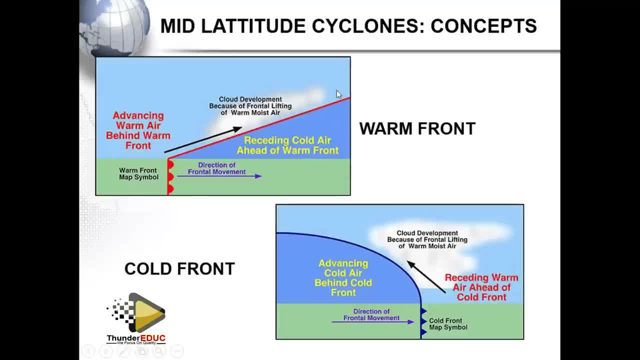 to be lengthened along the warm front, But these kind of clouds- karas clouds, nimbostratus clouds and ultrastratus clouds- But here you can see that it's a very long cloud that is growing taller, with a very flat base. 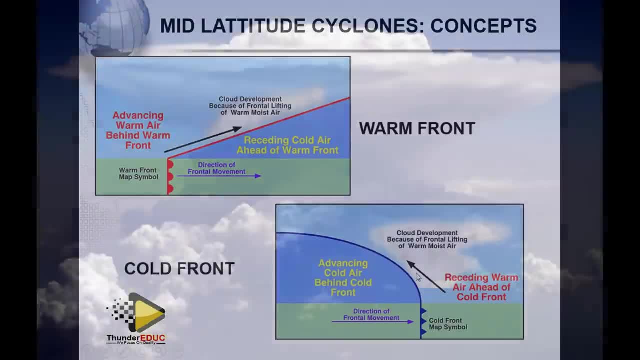 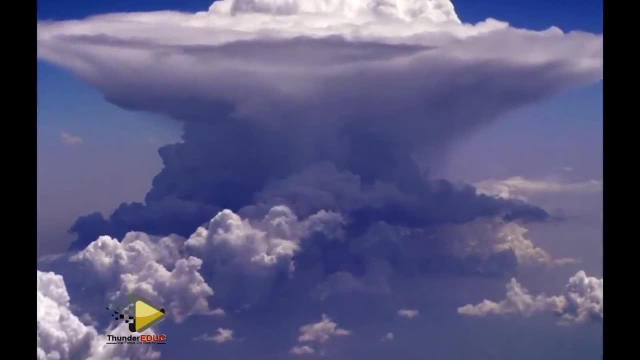 So these kind of clouds, what you call the cumulonimbostratus clouds, And these cumulonimbostratus clouds are basically associated with the following weather conditions like heavy rainfall, lightning, thunderstorms and, at times, hail. 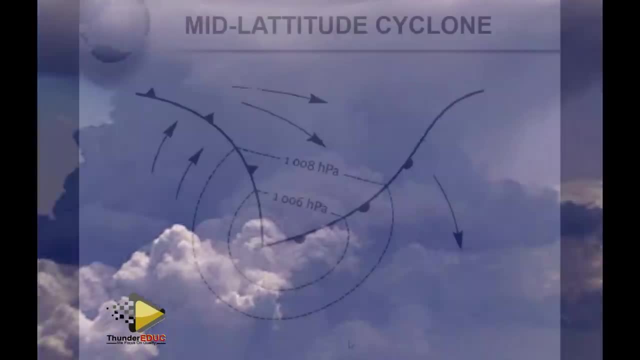 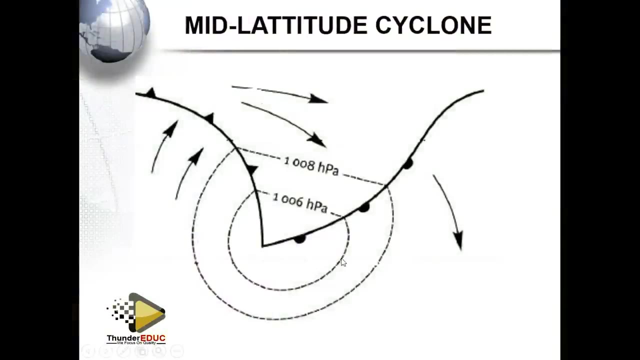 So that is what we refer to as the cold and the warm front, So those conditions are going to be prevailing there. So this is how a mediated cyclone will appear in the mature stage. OK, You can see the air rotating In that clockwise way. you can see the cold. 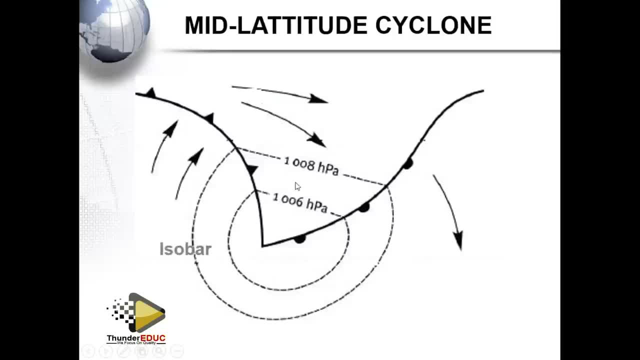 You can see the warm front. These lines here are called isobars because of this hectopascal, And then this one is called the cold front that is prevailing here. Remember we said the cold front basically is represented by these triangle symbols. 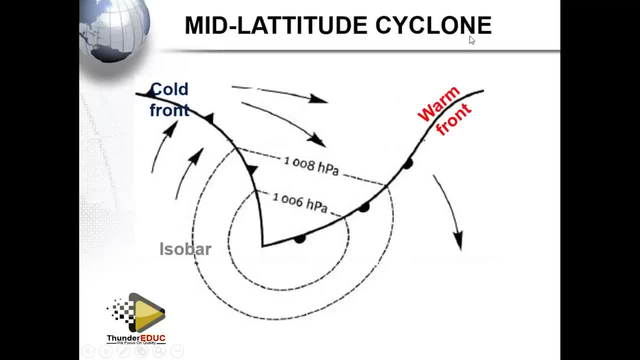 Then we also have a warm front on the other side. If you see critically, you'll find out that this warm front and the cold front are represented by different colors. Remember: warm it's going to be, red it's a bit hot. 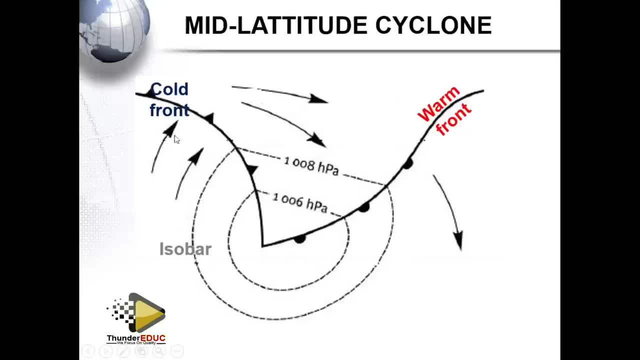 Then cold is blue because it is colder. But what is a cold front? by the way, We're talking about cold front, We're talking about warm front. What's a cold front? A cold front is just going to be a parcel of cold air. 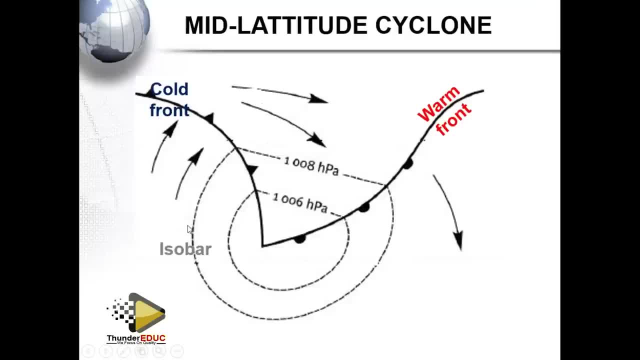 that is going to be separating the warm sector from the cold sector. It's going to be cold air alone, In other words, the edge of cold air that is pushing towards the warm sector. Then we have the warm front here, So it's going to be a parcel of warm air. 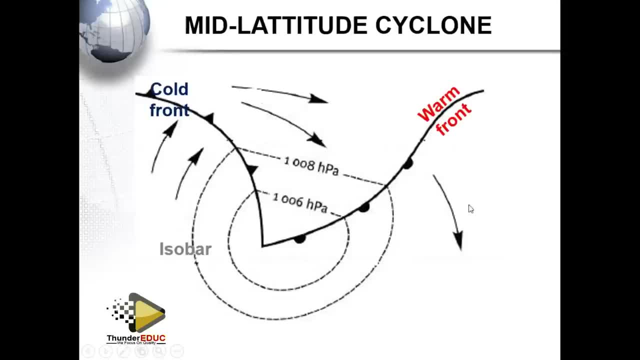 that is in the front of or that is pushing towards this other side. So it's going to be a warm sector, a warm front. So this is a parcel of warm air and this is a parcel of cold air. So in the center it's a low pressure. 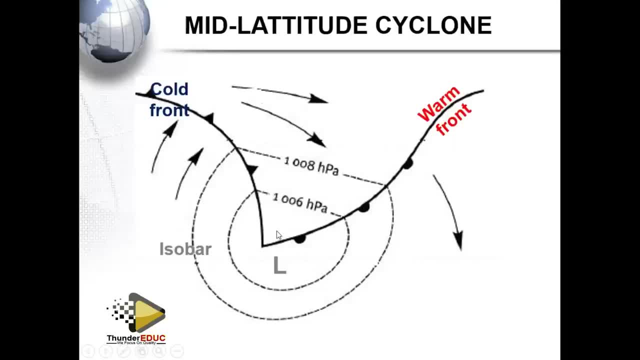 as pressure drops further down below 1,000 hectopascal. These arrows, we said It is, This part is representing the rotation of the saturation of A or the rotation of a cyclone. And we said in the Southern hemisphere it is rotating, lock wise. 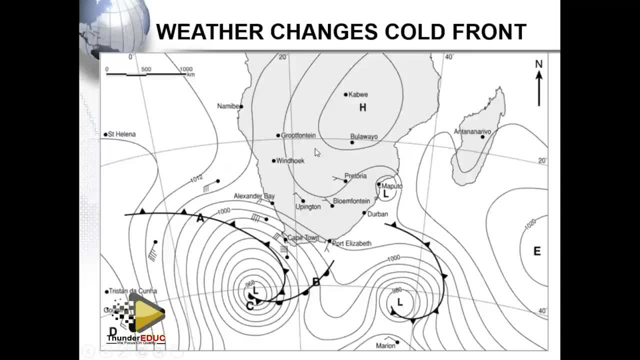 So the whole of this sector here that you see that it is, is going to be the warm sector in the whole of the sector at the bottom that is shaded with that kind of color is the cold sector. So the cold sector is covered in this whole section and the warm sector is covering that whole section. 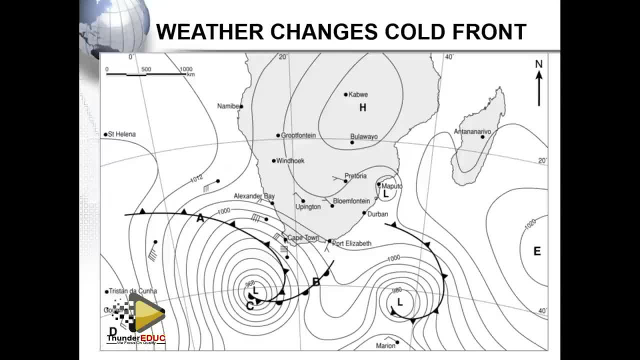 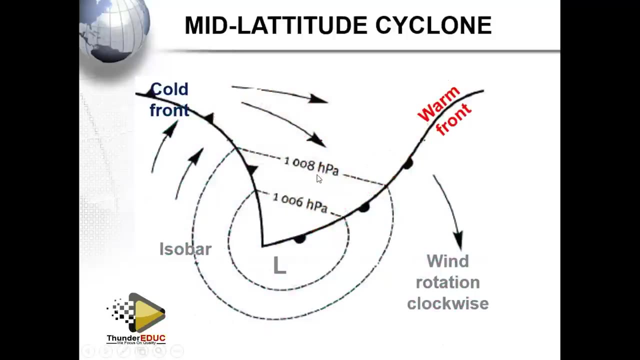 So that is basically explaining this: medicines, what we call the stages of the tropical, of a mid-latitude cyclone. hope, guys, we are understanding each other and you are moving at the same pace. okay, so now we must understand, uh, before we even move here, we must know- oh, i, i must explain this to you- that, uh, what happens when this cold front. 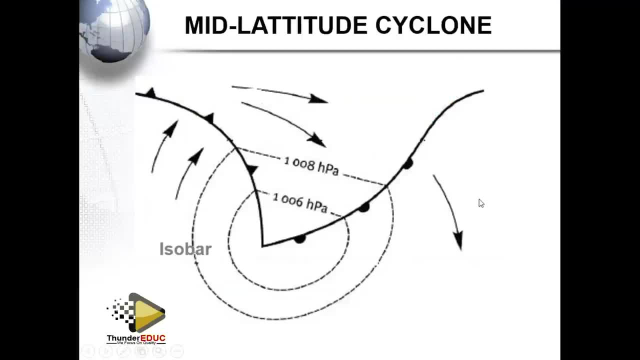 passes okay, or what happens when, uh, we reach the occlusion stage. you must know that when you reach the occlusion stage, the ground is going to be, for the warm air is going to be forced to move away from the ground and therefore the ground will be basically occupied by cold air. and therefore, what? 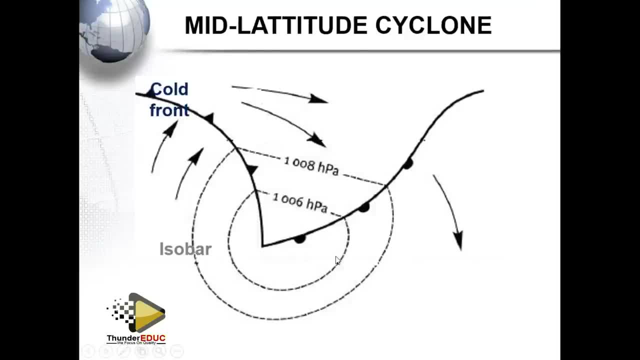 will happen. the air temperature is going to decrease as the cold air is basically passing in the same line. we shall see that in the, the air pressure is also going to rise, it's going to be high pressure and therefore we shall experience stable weather condition at that particular moment. so we need to look at this, this: 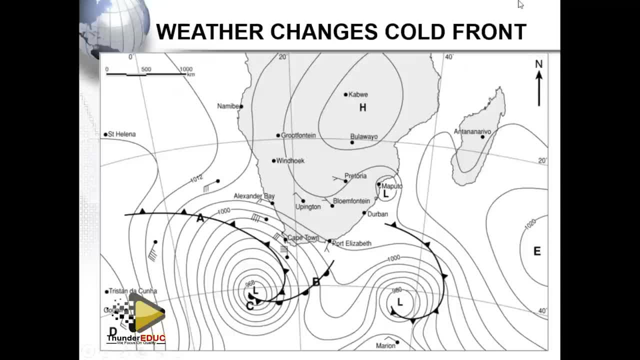 is a synoptic weather map, um, and i want us to look at it and critically, to see that. what weather changes are caused by the cold front? look at that, um, in this case, uh, on this way the map, we have to be analytical and analyze a lot of things when you see this weather map. 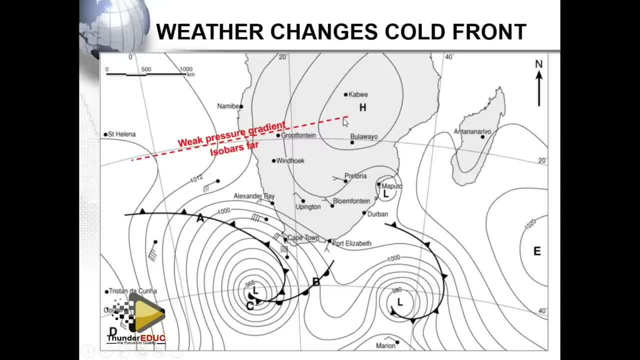 look at the isobars. here the isobars are far away spaced from each other. so because the isobars are having a very big space as you're moving away from each other, it means the pressure gradient is weak. but when it is like this, when they are so close, 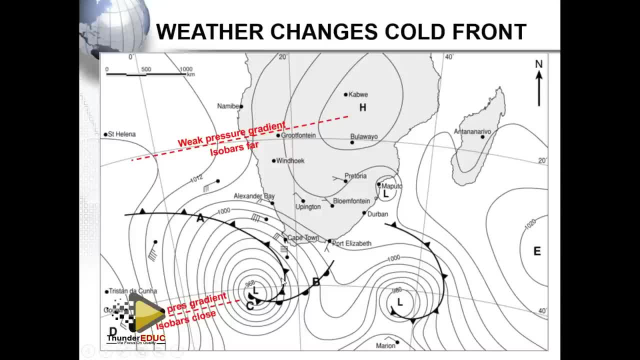 we say it is a steep pressure gradient because isobars are so close to each other. what is um the implication of this? it simply means if the pressure gradient is steep, the wind speed is going to be very high. here, the wind speed is going to be very slow. okay, this is the cold front here. 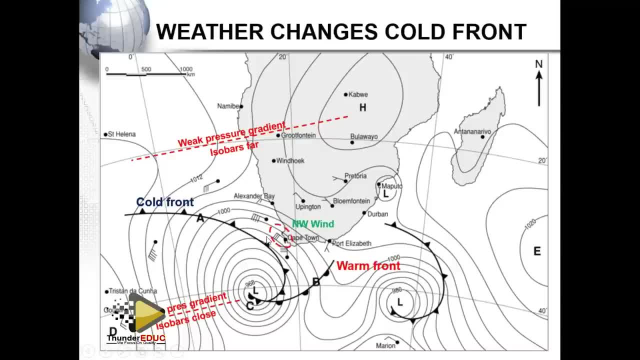 and therefore we also have the warm front there in the same line we have um this north northwest winds. look at this. these station models are showing us the wind direction. from the station model it is in the north or west direction. therefore we say the wind is rotating in that um northwest direction. then we also look here. 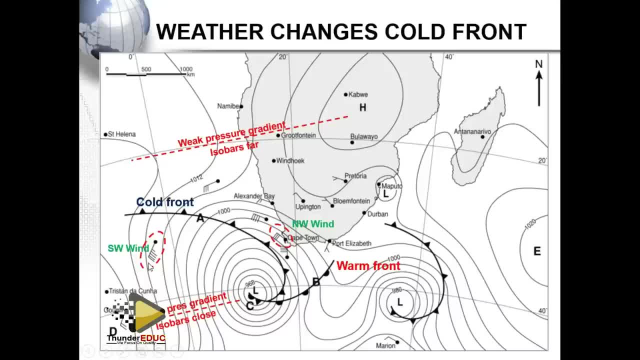 that, as it is coming here, it is in the southwest um direction. as you see, it's indicated by the station model. so, um hope, guys, you understand what we mean by station model. social model is just a symbolic element or a model that is used to explain um the weather. 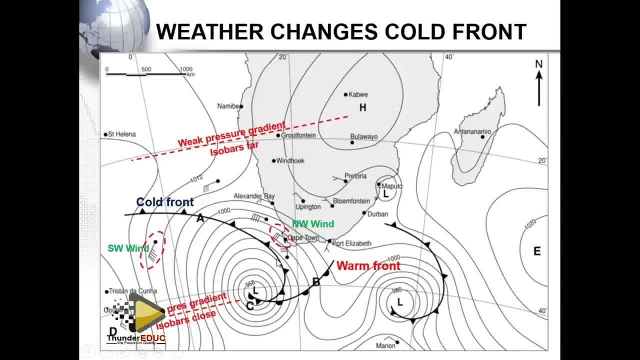 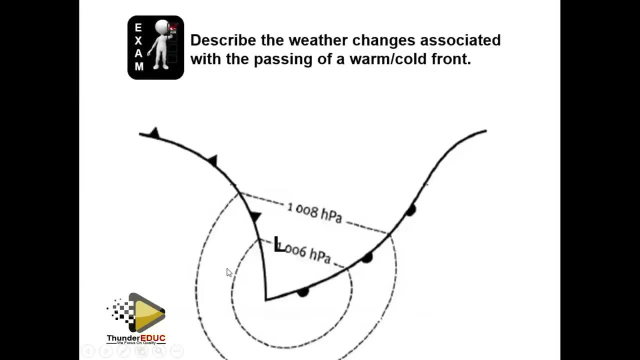 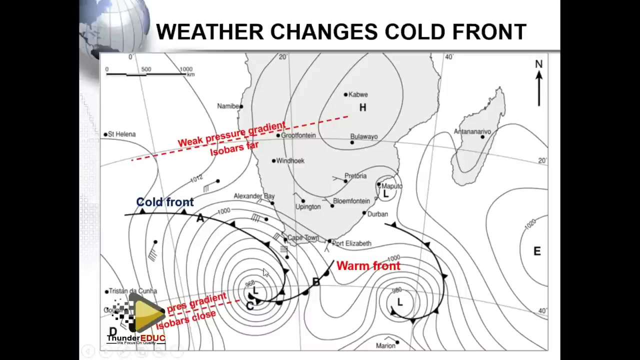 conditions that are experienced. so within here in the warm sector, um, the wind is moving in that northwesterly direction as it is depicted here, but here it is moving in the southwesterly direction as it is indicated today. okay, so in that case we have, uh, understood this, so we can see, remember. 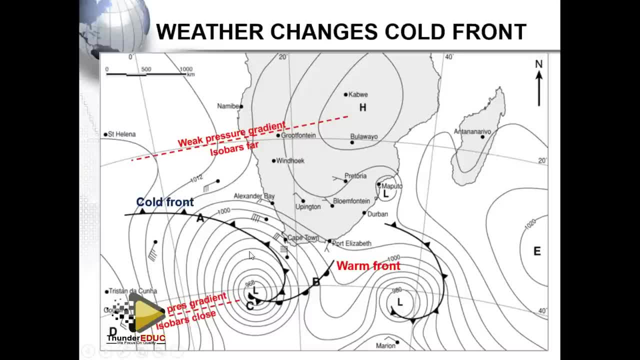 in our previous map, uh, synoptic weather map- we showed what we mean by families are the families whereby it is existing in series. so there is one here, there is one here moving in this western direction, and you must note we said also that cold different affects western cape during winter. what depicts the winter season here is that we have got a high pressure. 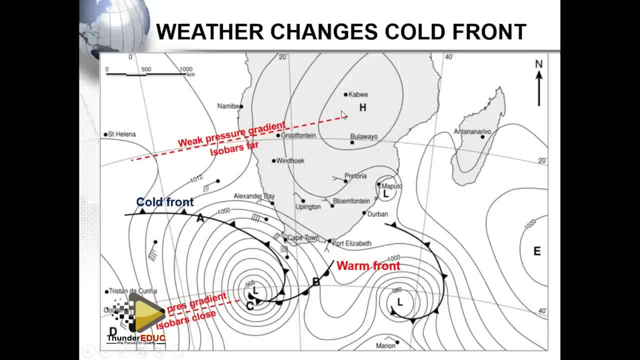 in the interior here. okay is a high pressure here in the interior which shows that it is winter in the interior here. so we can also look at um, um, the cold front it approaching um western cape. it approaches western cape basically during the winter season, but remember we said it's uh, occurred throughout the year. 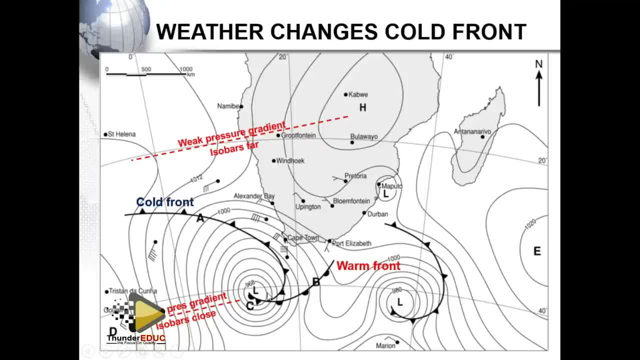 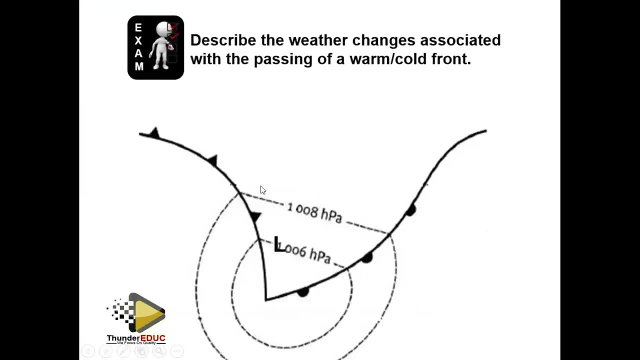 therefore, what happens is that it's it's winter, it is close to south africa and therefore, if it is summer, it will move far away, further south away from um south africa. okay, so we move forward. we need to understand now some of the examinable questions, or some of the questions that are likely. 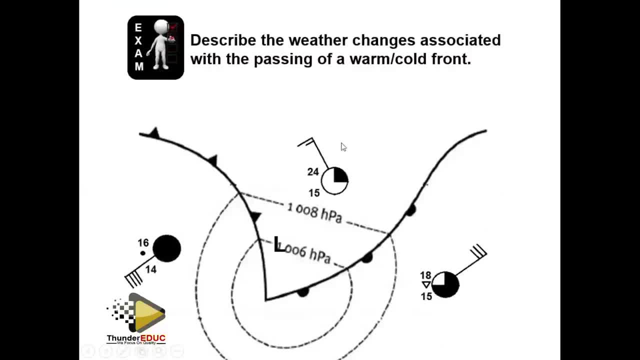 to be said. what have we looked at? we have looked at all those ones. we have looked at the cold front, the stages of the development, the initial stage development stage. we have looked at, uh at um, the weather conditions that are experienced when the cold front has passed, and so on and so forth. 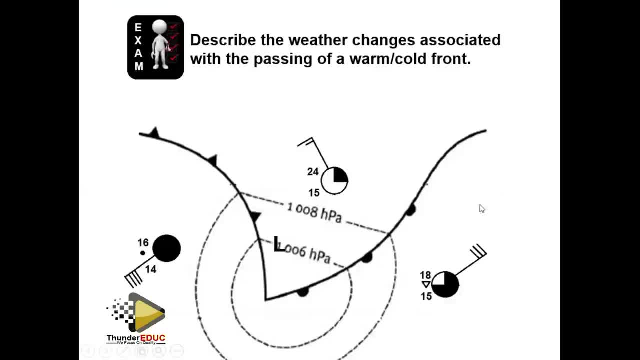 so we need to see, if they tell you to describe the weather, uh, the weather conditions that are experienced here. what do we use? we use the station model and this station model is clearly depicting the conditions you see here in the warm sector, the wind is, the wind direction is not waste here. we said it is south west, okay. 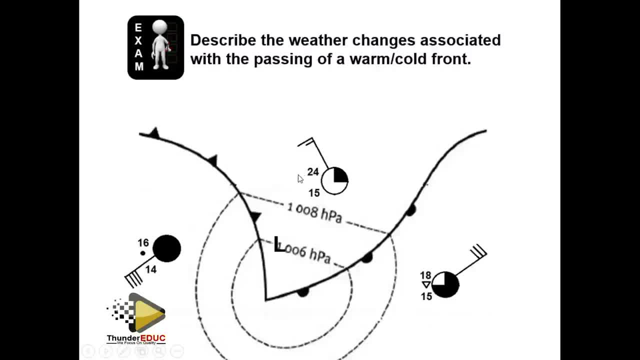 this number above. here is the air temperature, which we could say that the maximum temperature, therefore temperature within the warm sector, is 24.. Here the minimum is 15.. Here, where we say that this zone here is a cold sector that is occupied by cold air. therefore, you can also look at this. 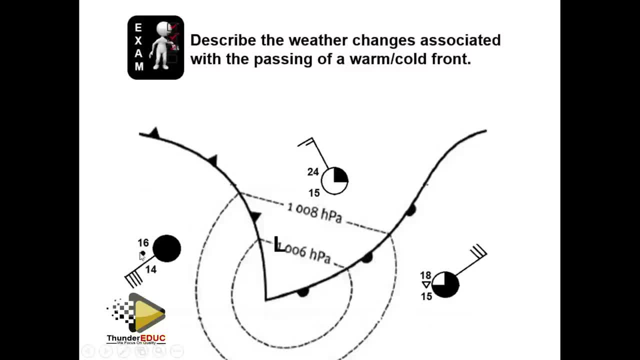 and you see that this one is 16,, this one is 14.. This way is a bit colder than what will happen here. So at the warm front temperature rises to the maximum. okay, So that's why you see the the temperature here is 24 and 15.. The difference is also not that big, but when you come here, 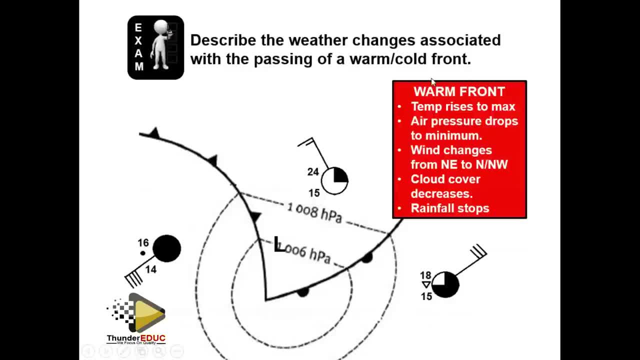 it is 16 and 14, which is a bit lower than what is happening here. So in the warm front, air pressure drops to the minimum. We mean air pressure, atmospheric pressure drops. Why is it dropping? It is dropping because within this sector it is rising warm air As warm air rises. 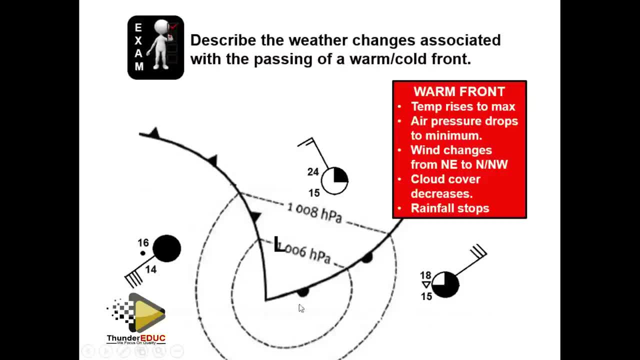 above or as warm air rises into the atmosphere, the ground or the surface of the air is going to drop. So when you come here, the temperature here is 24 and 15.. The surface is left with low pressure. That's why we say the pressure drops to the minimum. 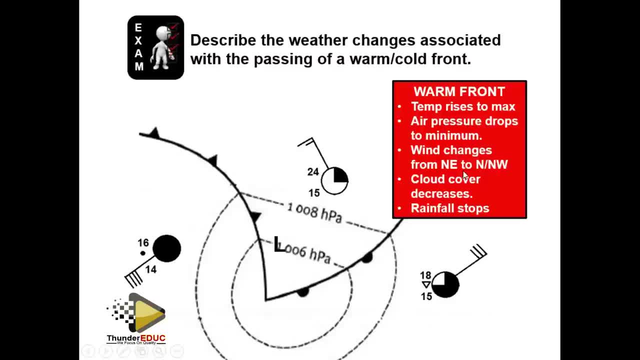 So wind direction changes from northeast to northwest or the northwest direction, as it is depicted here on the station model. So it will change. Remember it is rising like this, but the rotation is this other side, As it is rotating like this, but this warm air is in. 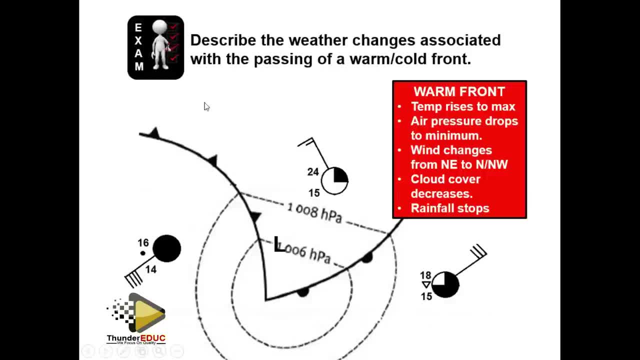 position to rise like this. So it is going to result into this wind to move in that north and northwest direction. The cloud cover is also going to decrease. Okay, cloud cover is going to decrease. Why is it decreasing? Because within this sector, the warm air is rising. Therefore, 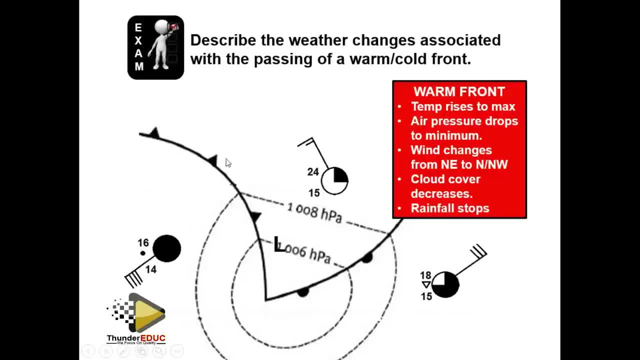 it's going to be in position to force its condition to be formed along the cold front, not at the warm front. Therefore, at the warm front because here warm air is rising on this other side. Here we shall have kind of clouds like limbo stratus, the karas cloud. 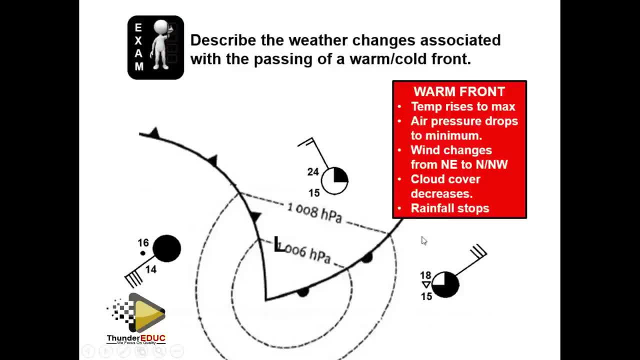 and ultra stratus clouds. Therefore, even the rainfall will have to drop. Why? Because there is no rising warm air. Remember, rainfall only forms when the warm air rises, condensing in the upper atmosphere to form clouds. Okay, look at the cold front Here, the conditions we explained. 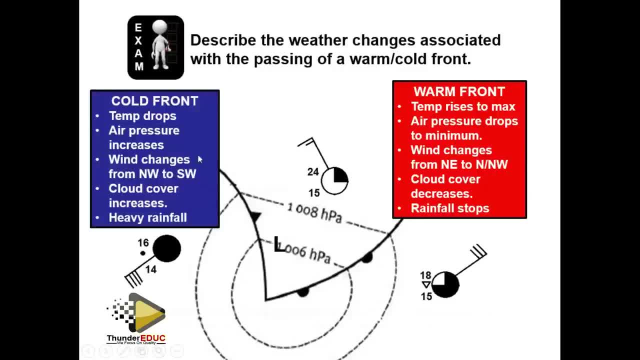 are on the warm front, this front here, So we need to explain what happens on this cold front. On this cold front, temperature drops. It's cold, It's the cold air that is approaching on this other side. Therefore, the temperatures are going to go further down. The air pressure is going to increase. Remember. 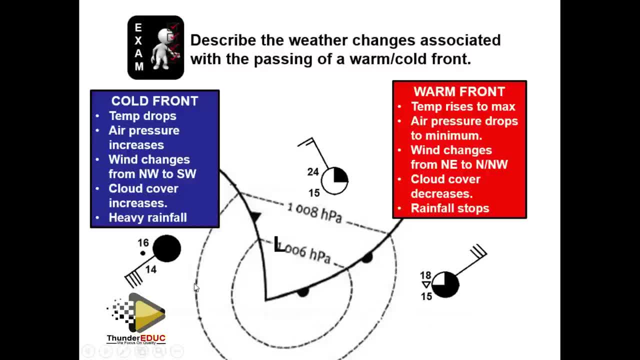 your basics. We say that if it is cold, pressure is high, If it is warm, pressure is low. So in this case, because we're experiencing very cold conditions, or cold conditions on this other side, therefore, the pressure will have to drop further. 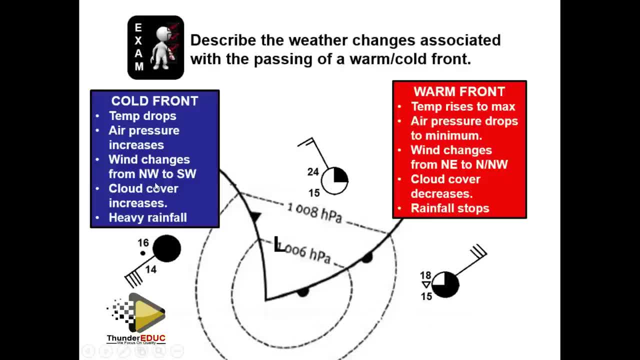 But this forms because the wind will move down, or the down that you enjoy hearing. Instead, the one that was moving here in the northwest direction is going to move in the southwest direction. So it will be because of what you call the backing, or that is what you call backing. 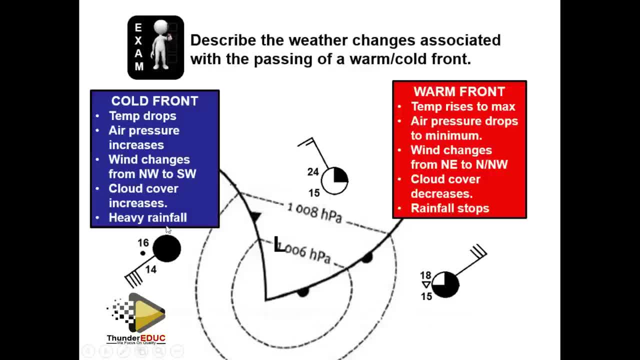 Backing simply means the change in direction within these sectors. We have a plot cover and increasing cloud cover is increasing. Why is it increasing? There is a rising warm air So tall Elementary-adores prices. that is going to resolve into that. Nevada crisp 49 direct from. 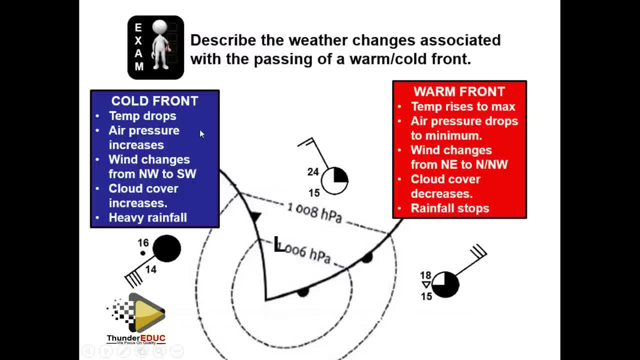 each side toойти to gather meat- 3% from each site down, Okay, into that wide base, tall clouds along the cold front. we also have heavy rainfall. remember the moment we talk about those clouds, those big clouds that develop. they come with heavy rainfall okay. 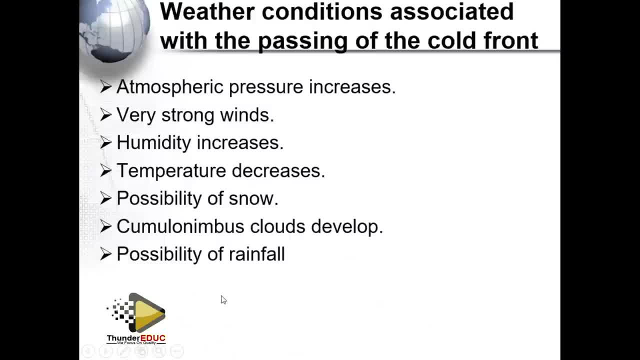 that is what we refer to as uh, the weather conditions, so that the weather conditions are experienced on the cold front and the warm front. we also look at the weather conditions associated with the passing of the cold front after it has passed, i think on very many occasions. 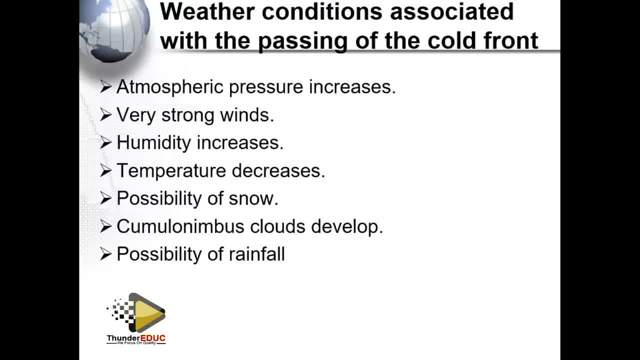 in south africa. you've been warned. when on the radio stations or tv stations that the cold front is approaching south africa, please wear warm- meaning that you are going to experience very cold conditions, heavy rainfall and so on and so forth. the same way, after it has passed, it causes 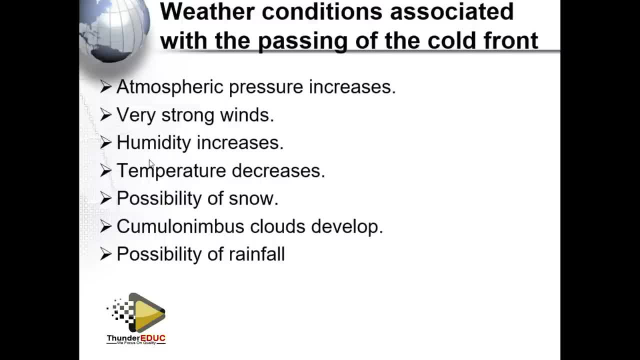 some conditions that we are looking at right now. for example, atmospheric pressure increases. why is it increasing? it is increasing because the cold front is passing. remember we said: behind the cold front is called a. that means as the cold front passes, the cold air is following that cold. 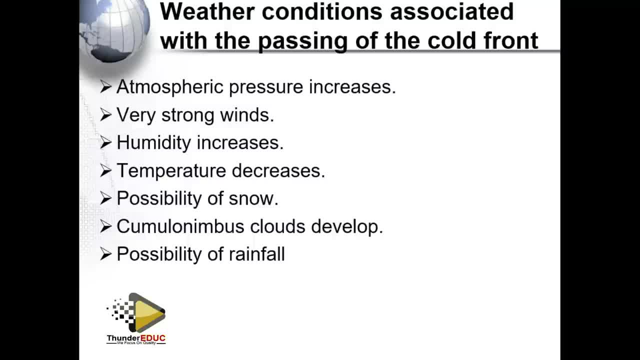 air is going to result into the area being occupied by cold air and that will result into the draw resulting into dropping of the pressure pressure. the increasing of the pressure pressure is increasing because the air is cold as it is descending onto the earthy surface, it will increase. 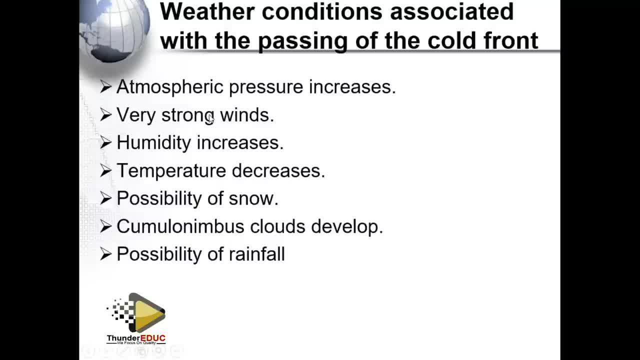 exactly more pressure onto the earthy surface. we also have very strong winds. these winds are existing because the cold front is passing, so it will be followed with very strong, strong winds. remember we said that the cold front and um, this system is associated with a steep gradient. 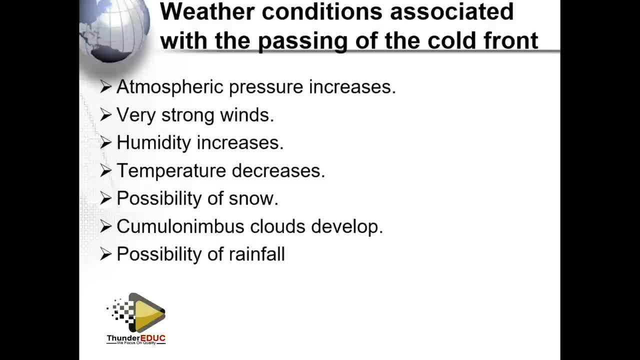 as i indicated to you there, and i say the steep gradient results into the winds to move or to to grow very fast. then humidity increases. why is humidity increasing? humidity, remember humidity, we say, is the amount of water vapor in the atmosphere. so when the cold front passes, remember it will. 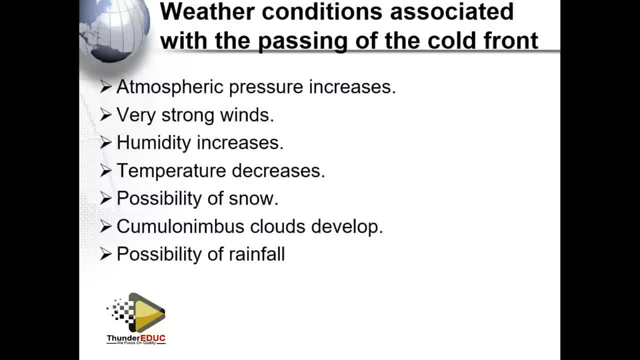 result into with increasing. why is it increasing? it is increasing because there is rising warm air along with the cold front, so that rising warm air it is warm. remember, warm air is moist. okay, it is moist because it is moist. it has got all our moisture embedded in. that goes into the atmosphere to increase the humidity. 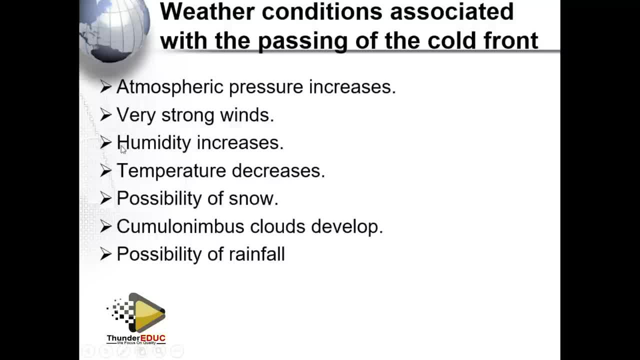 we also have temperatures decreasing. temperatures are decreasing or the air temperatures are decreasing because of the fact that the cold conditions are now prevailing. there is a possibility of snow as the pressure or as the temperatures drop further, further, further down. it means it can go um to even 0.0 degrees, to even minus. therefore, we shall 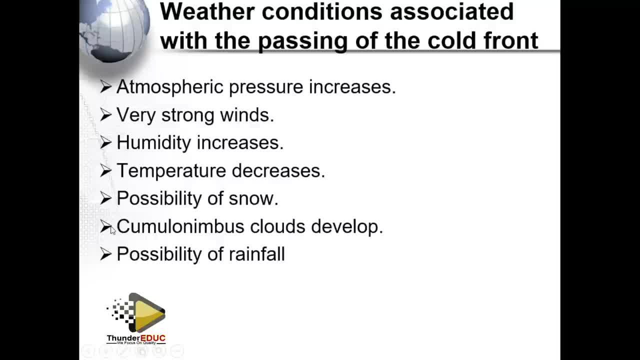 end up experiencing snow. cumulonimbus clouds form. why cumulonimbus clouds form? they form because there is continuous rising of warm air along with the cold front. so when there is that rising of warm air, it will result into the development of cloning mass clouds in the upper atmosphere. 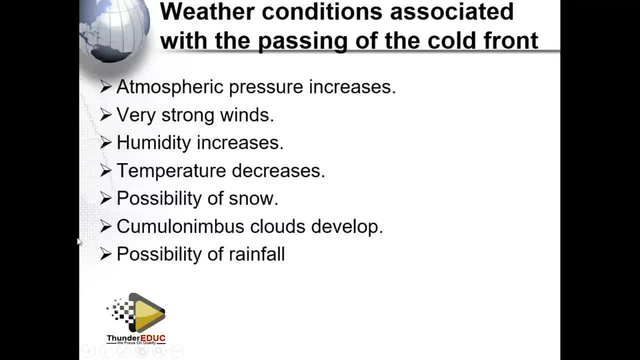 and therefore cumulonimbus clouds are associated with it- rainfall. that's why we say there is a possibility of rainfall. that is not only. we also see that. uh, besides that, cumulonimbus clouds are associated with the thunderstorms, lightning, hail- all those weather conditions are going to be prevailing, okay. 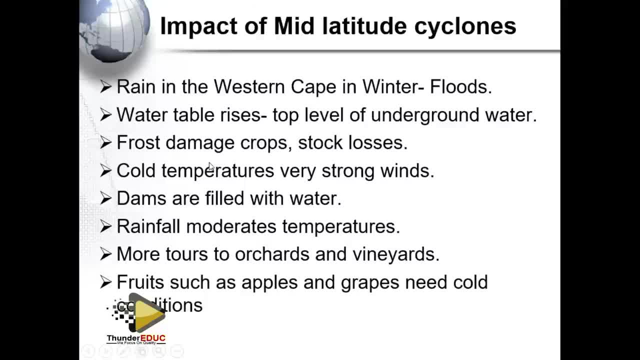 so, when this weather condition prevails, what is going to happen? we need to know that this mediate cyclone, after it is affecting south africa, it will have an impact to the people, to the environment, to the, to the area where it has passed or where it is prevailing. so what are these impacts? the 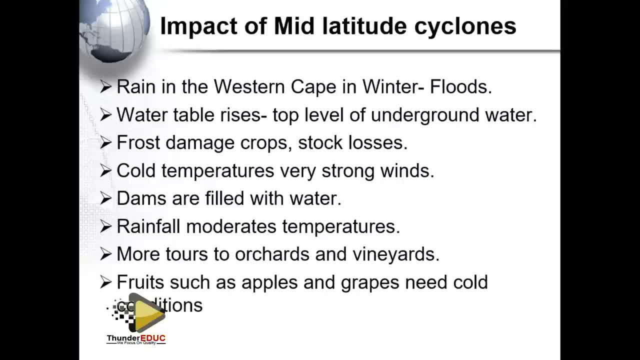 impacts of immediate cyclone are here. number one: rainfall. we have just mentioned that the cold front has got conimbus clouds that will result into rainfall. this rainfall is forming in winter. that's why, you see, western cape is experiencing most of its rainfall in winter. however, this 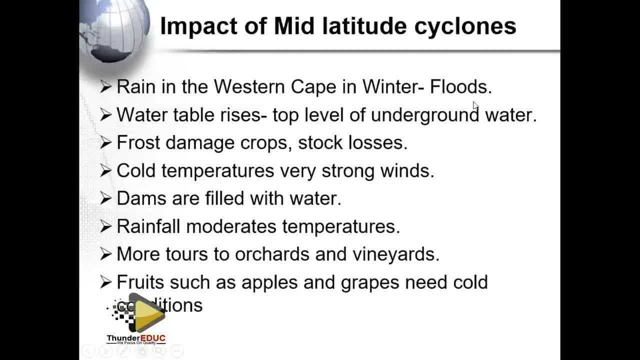 heavy rainfall sometimes results into floods, and floods are likely to uh wash away vegetation, which is an environmental effect. these floods are likely to come to to disorganize the ecosystem. these floods are likely to damage the infrastructures, roads and bridges, and so on and so forth. therefore, you must understand, learners, that this rainfall that 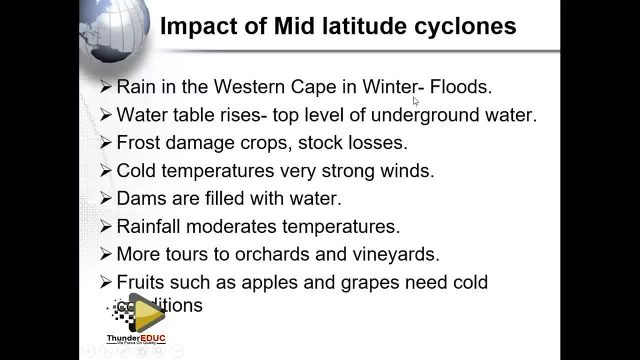 are caused by a military cycle. sometimes it is good for the winter plants, but sometimes it's bad for sometimes too much flood that are going to result. okay, it depends on the nature of the question that is asked, so that you can handle it or tackle it in that way. it also increases the water table. what is the water table? water table is the. 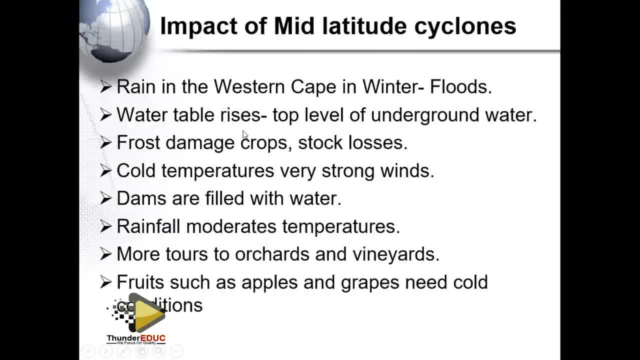 uppermost limit of the water underground. so it is going to increase. as it rains water sips underground. that infiltration of the water underground it results into the underground water to increase which rises the water table. so when the water table rises it will mean that the level 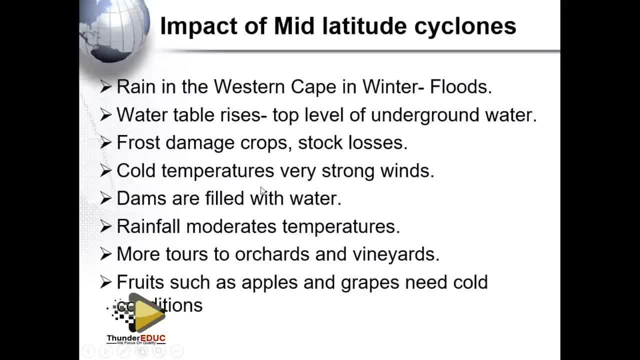 will also increase. so to those people who are interested in drilling boreholes, they can easily access the water, the rivers that are flowing over the area where the water table is across the earthy surface, those rivers will have ever water flowing because they will have continuity of water. 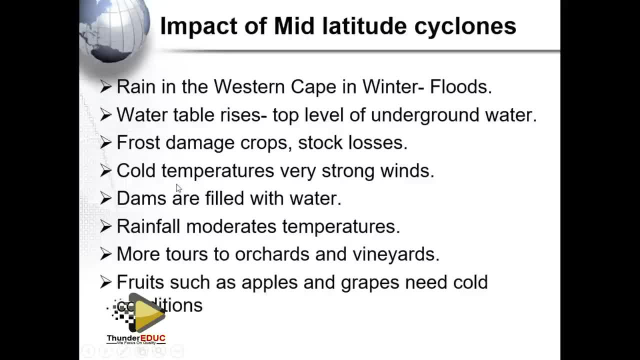 from the underground. so we also know that we said that it is associated with a very, very cold condition to sometimes leading at times leading to snow, so the frosts are likely to form, which will damage the crops and therefore it will result into losses to farmers, who are basically growing. 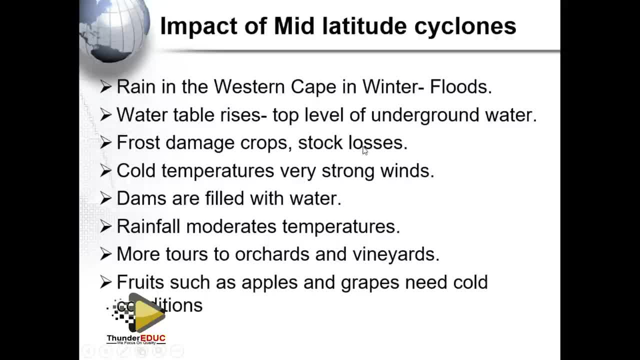 winter crops. that is it's going to. that means it's going to negatively affect the farmers. we also know that cold temperatures are very, very strong. uh, cold temperatures are going to exist and therefore these cold temperatures are also coupled with very strong winds. you know it's called strong winds. you'll find that trees are uprooted. 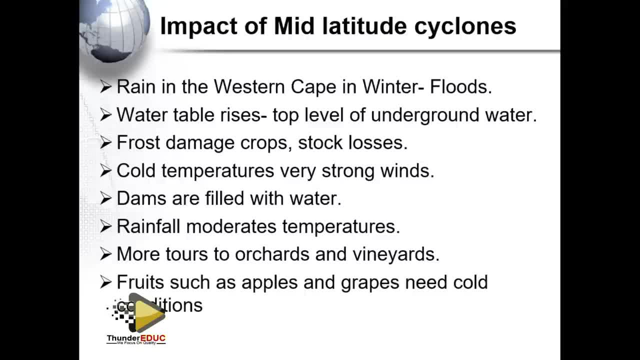 buildings are put down, bridges are damaged- all those ones are going to come because of the strong winds and these cold temperatures. sometimes they become unbearable to people. sometimes it even causes wastage of electricity, because people have to make means to cope up with the existing environment. therefore, they will put on heaters that will consume a lot of electricity, ending up. 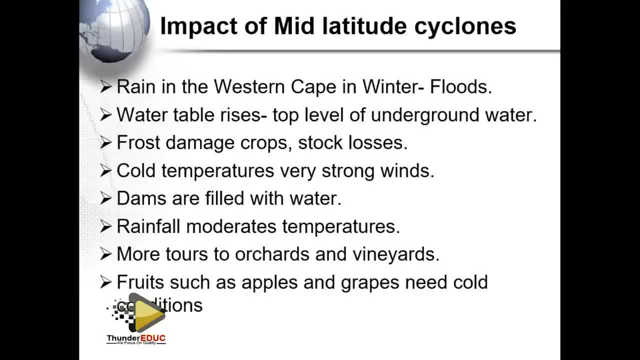 in grazing bills for people. it's a negative impact. okay, we also know that dams are going to be filled with water. this is going to be positive because when dams are having water, that means farmers will need water for irrigation. other places where they will need water for industrial use, they can.